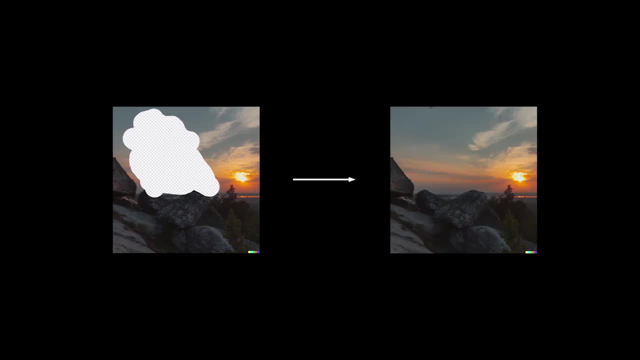 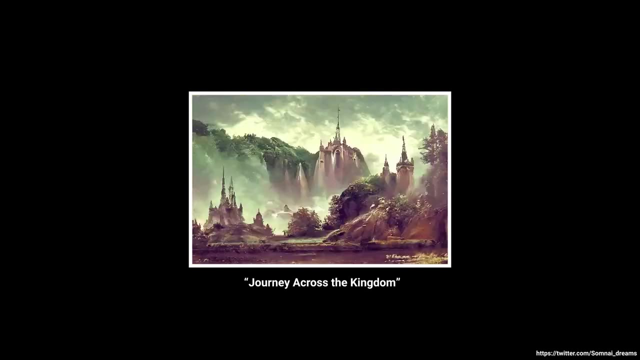 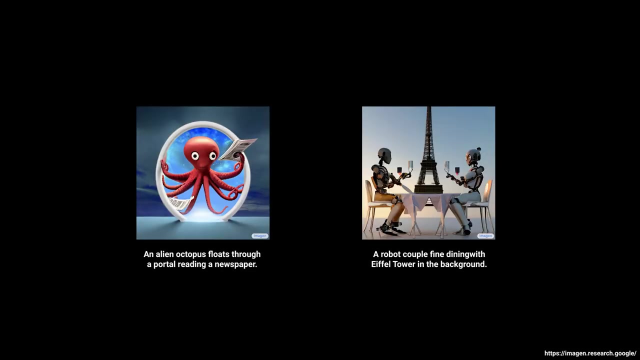 and then asked to remove the tree, and this is the result. Just amazing. With other models, like disco diffusion, you can even create little animations, given a text prompt. So you see that these models are capable of creating incredible results and it's so much fun to play around with them. So, without further ado, let's try to 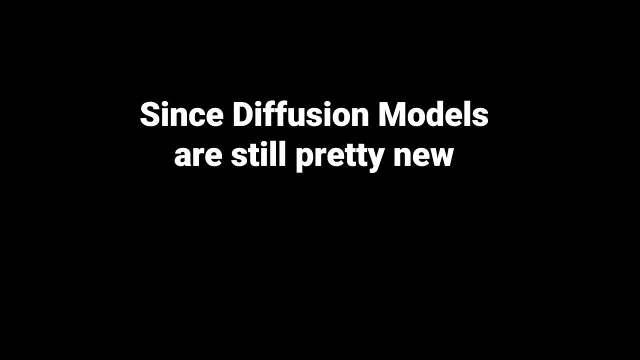 understand them. Since diffusion models are still pretty new in the image synthesis regime and the number of relevant papers is not too big, I want to cover the most fundamental papers in the image synthesis regime, So let's get started. First of all, the most basic fundamental papers about DDPMs, which led to the rapid 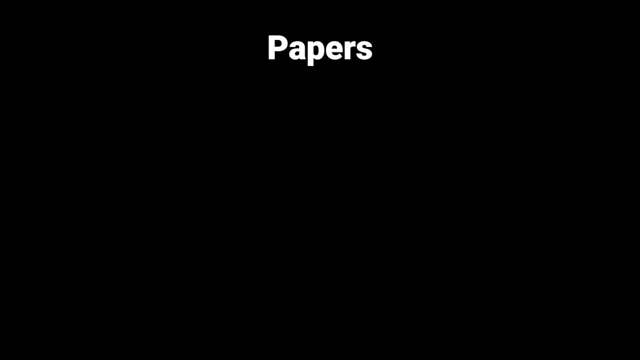 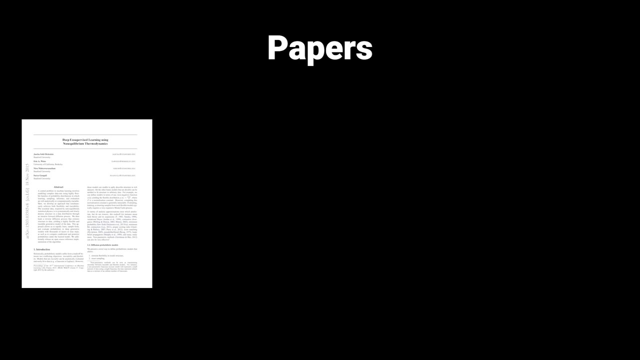 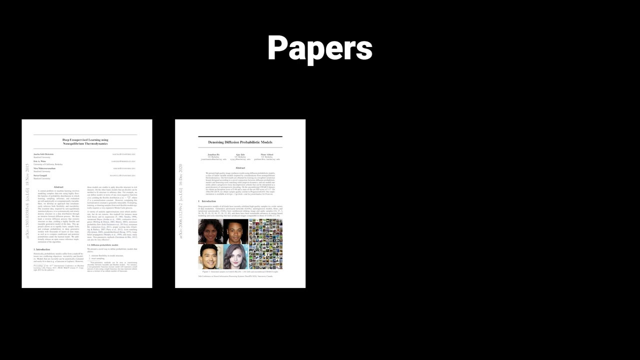 improvements for this technique in this video. Specifically, I want to talk about the following four papers. First of all, the original paper from 2015, which introduced this technique to the field of machine learning, coming originally from statistical physics. Then, five years later, the second influential paper was: 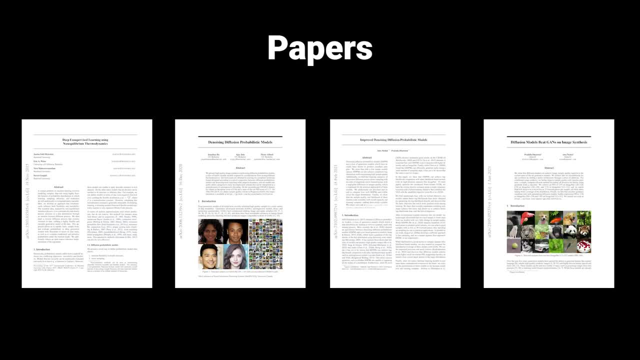 published and introduced a few groundbreaking changes which led to a huge jump in quality. After that, two researchers from OpenAI took on the stock of these papers and ended this technology challenge and introduced even more improvements in two consecutive papers in 2021, which resulted 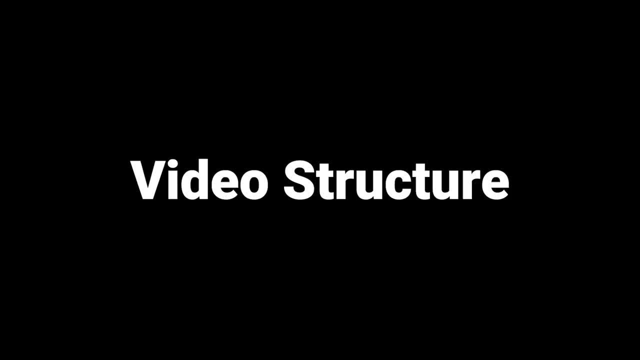 in better performance and faster runtime. The video will be structured as follows. I will be first talking about the general idea of diffusion models, how they work, and why they work. I will try to do this on a really intuitive level, without too much math involved. After that we'll be diving. 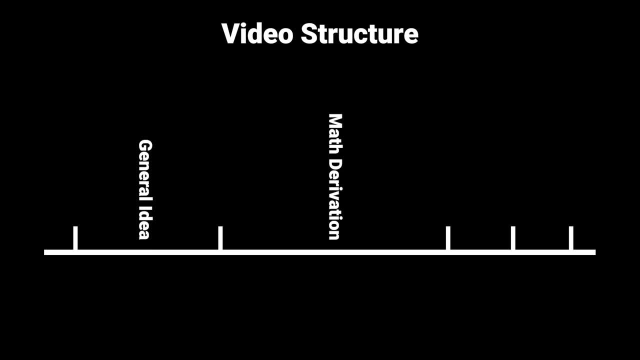 into the evil looking math formulas and, along with the pre-built intuition, I will try to explain the math behind DDPMs. Moreover, I will also be mentioning the different improvements which came from each of the four papers. Oh, and one side note. please forgive me if I won't be going into 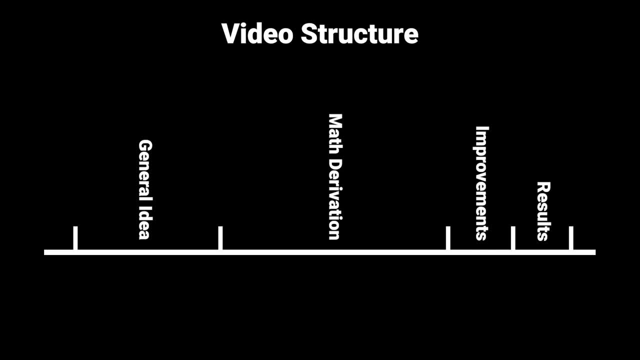 every single formula in detail of each paper, since this would go beyond the scope of this video and would explode the video length, And also feel free to use the timestamps in the description to go to the part which you are most interested in. So let's try to understand the idea. The 2015 paper. 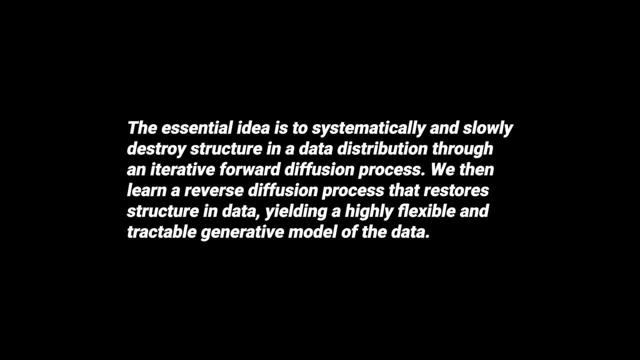 described the diffusion model as the following: The essential idea is to systematically and slowly destroy structure in a data distribution through an iterative forward diffusion process. We then learn a reverse diffusion process that restores structure and data, yielding a highly flexible and tractable generative model of the data. In short, 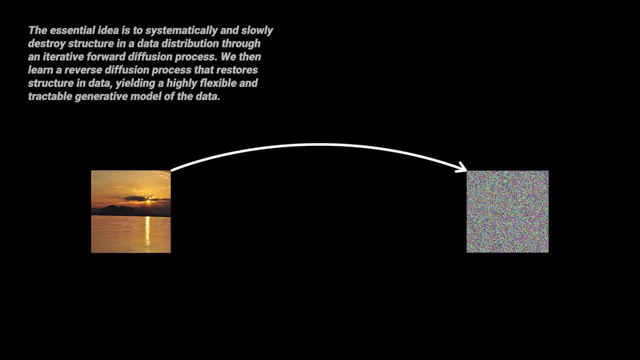 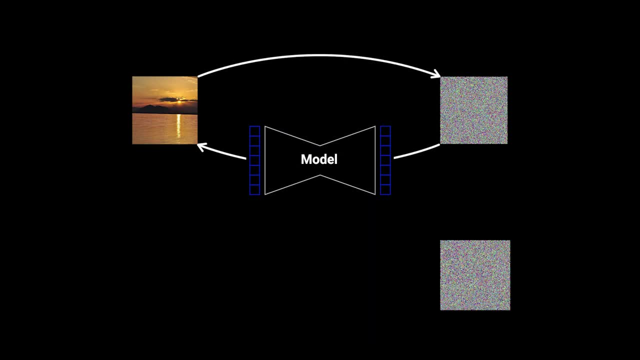 we apply a lot of noise to an image and then have a neural network for removing this noise. The idea now is, when the network for removing noise is learned properly, we can start off with completely random noise and let the model remove noise until we have a new image which could occur on our 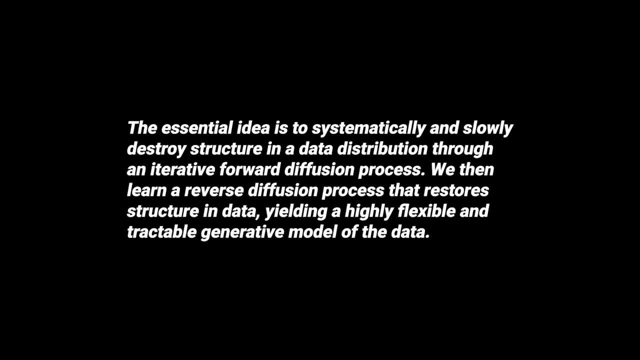 training data. To better understand this, let's take the previous statement apart. The authors talk about the forward and the reverse diffusion process. The forward diffusion process is applying noise to an image in an iterative fashion, So we start off with the original image and, step by step, add more. 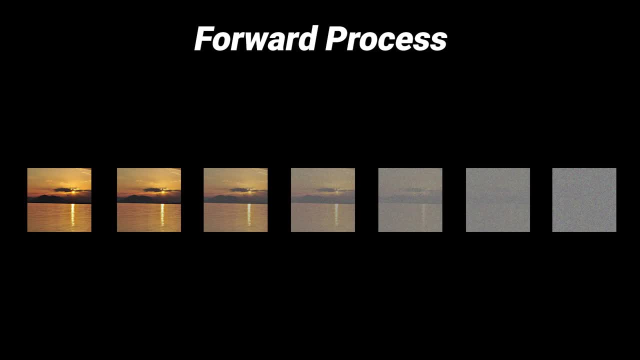 and more noise to the image. If we repeat this for a sufficient number of steps, the image will become pure noise. from 2015 decided to sample the noise from a normal distribution and this was not changed by any of the follow up papers. The authors showed that the image will converge to noise, which follows the noise distribution. 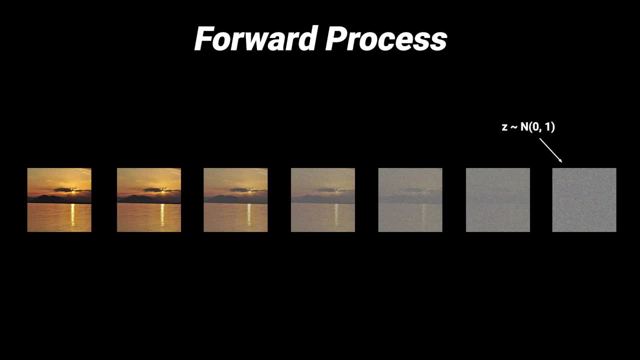 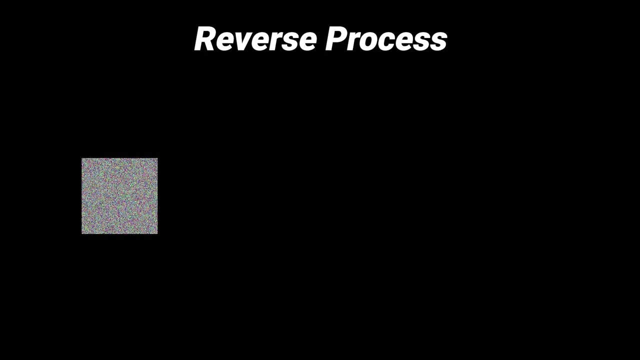 In our case, the image will turn into one which could come from a normal distribution. So we see that going from an image to noise is fairly simple. But what about learning the reverse and going from just noise to an image? This is what the authors call the reverse diffusion process, and it involves a neural 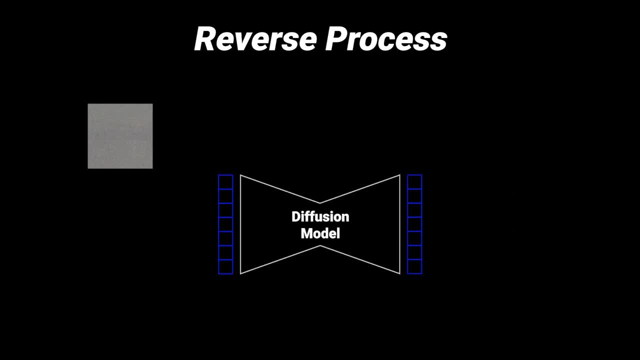 network learning to remove noise from an image step by step. That way we can give our model an image which just consists of noise, sampled from our normal distribution, and let the model gradually remove the noise until we have a clear looking image. And if you are wondering why we are doing this stepwise and not going from noise to 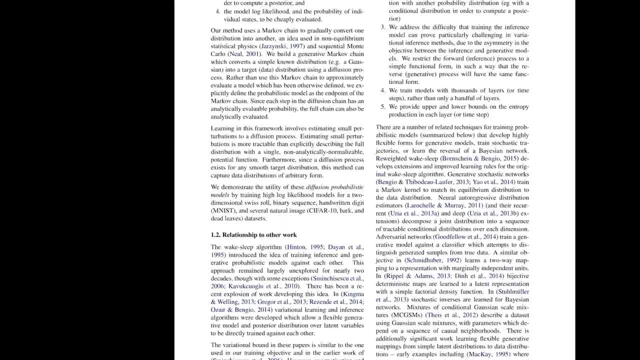 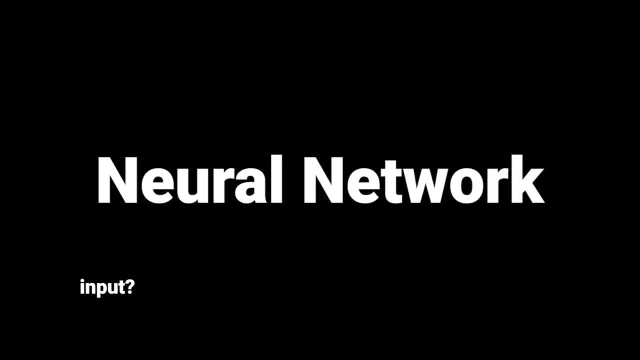 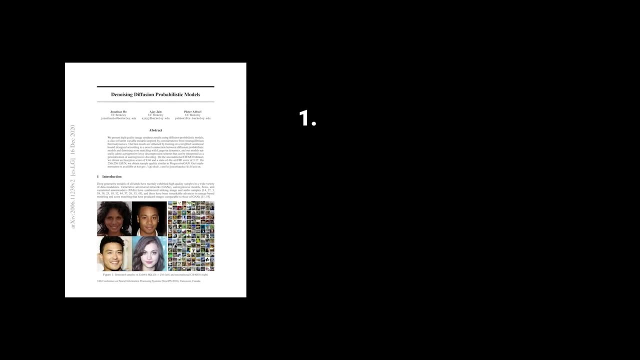 clear image instantly. the 2015 authors claimed that this approach would not be tractable and lead to much worse outcomes. So how does this neural network look like? What will it take in and predict eventually? The DDPM paper from 2020 laid out three things the network could predict. 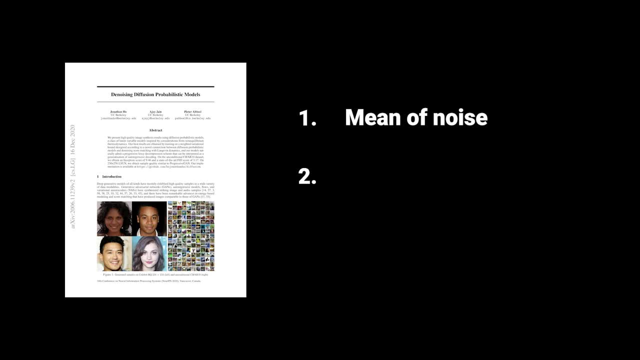 First, predicting the mean of the noise at each time step. Second, predicting the original image directly. And third, predicting the noise in the image directly, which could then just be subtracted from the noised image to get a little bit less noised image. We already said that predicting the original image won't work well, so we can ignore this. 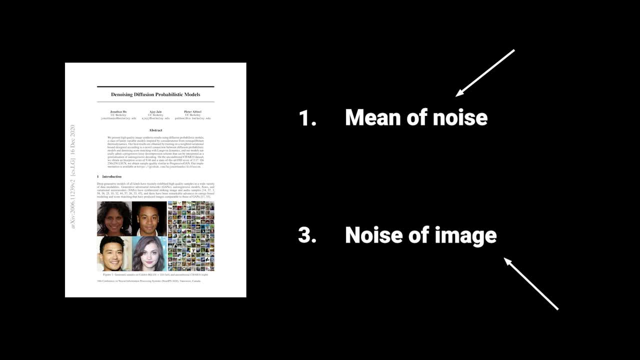 choice And, as you will see later, the first and the third option are the same, Just parametrized differently, And all authors decided to go with the third option and predict the noise directly. You may be wondering: why do we just predict the mean and not the variance in the first? 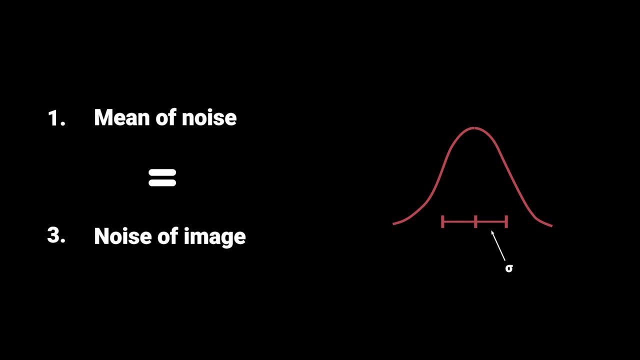 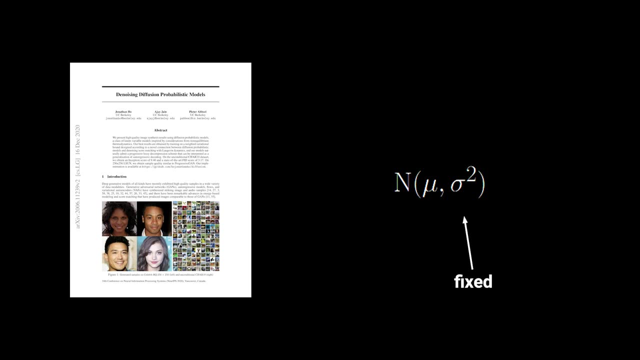 option A: normal distribution needs mean and variance. Well, the authors of the 2020 paper decided to fix the variance, and thus there is no need to predict it, since it's always readily available. I'll show what they fixed it to in the math part. 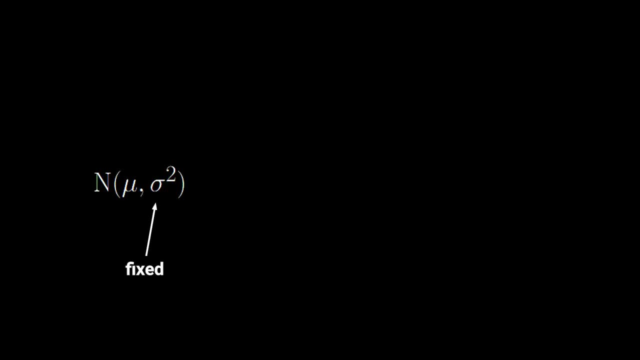 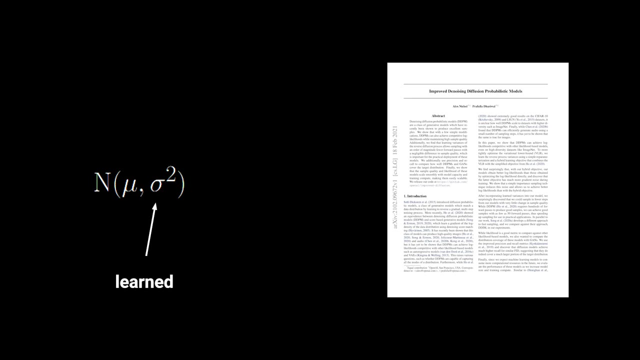 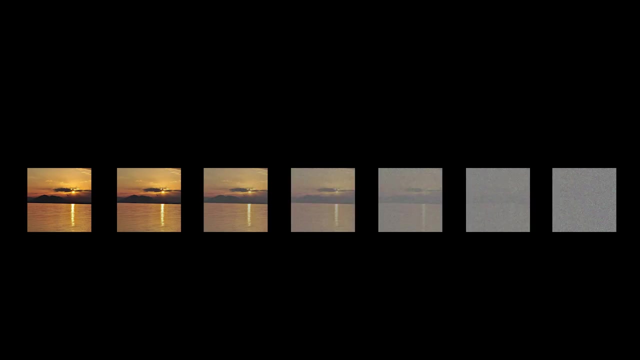 And later the choice of fixing the variance was rethought by the OpenAI organization In their first paper. they eventually decided to learn the variance too, because it would lead to improvements in the log likelihoods. But more on that later. Also, one more thing to note is that we don't employ the same amount of noise at each time. 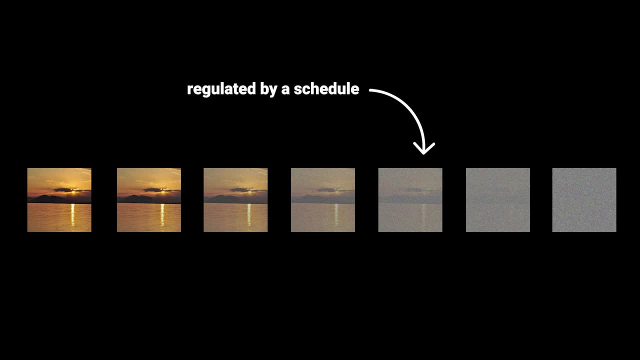 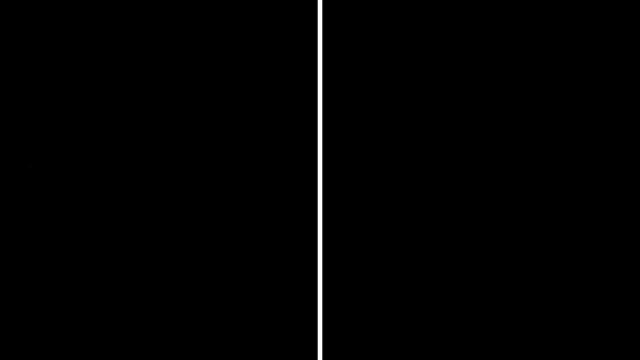 step in the forward process. This is being regulated by a schedule which scales the mean and the variance. This ensures that the variance doesn't explode as we add more and more noise. The paper from 2020 employed a linear schedule. Again, more on that later. 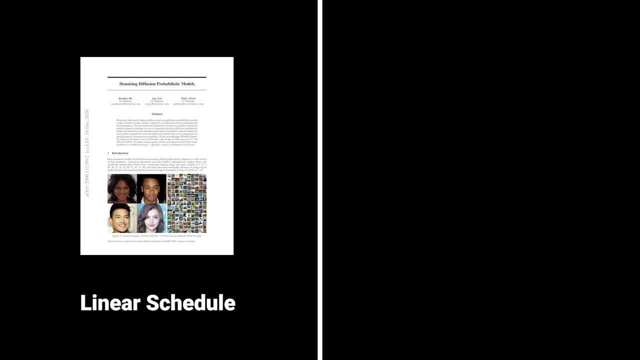 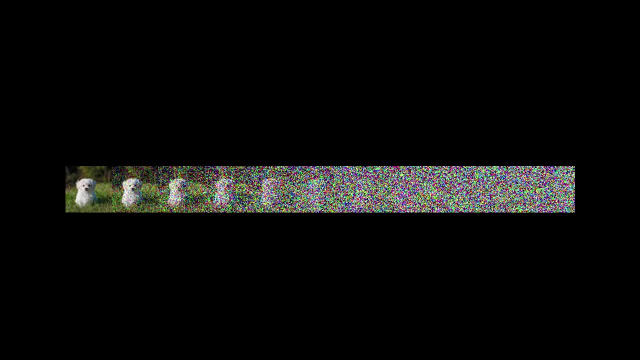 But to give you some intuition, If we apply the schedule to an image, the transformation would look like the following: Looking at that, the authors from OpenAI found this approach to be suboptimal, especially at the end of the noising process, Because you see that the last couple of time steps already seem like complete noise and 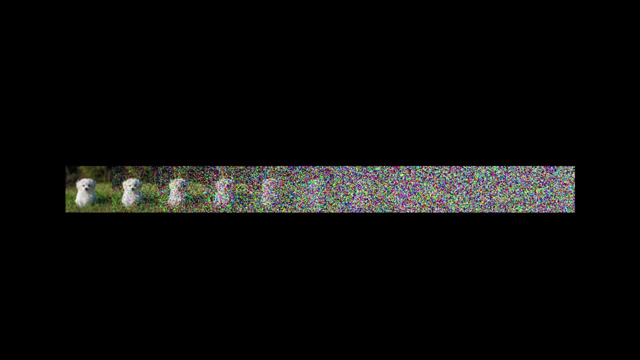 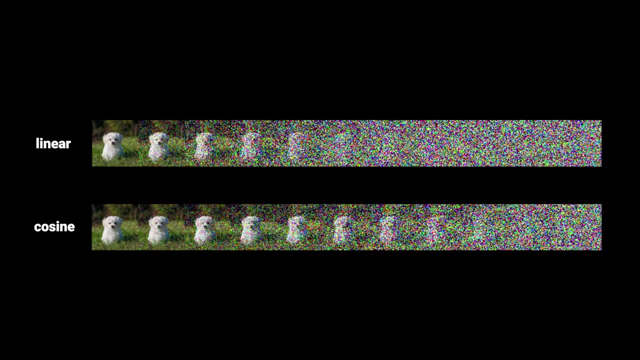 might be redundant. Also, they found that the information would be destroyed too fast. As a result, they created their own, called the cosine schedule. In the following image you can see the difference between both schedules. The cosine schedule destroys the variance. The cosine schedule destroys the information more slowly and solves both problems of the 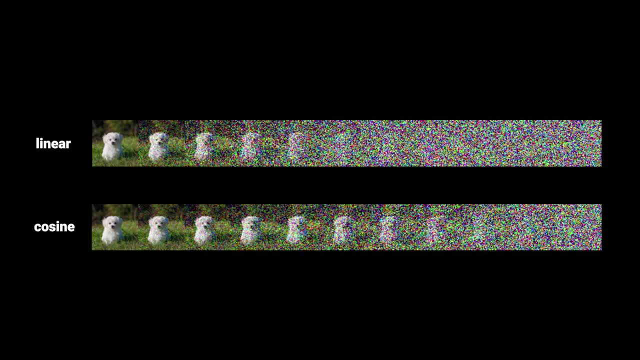 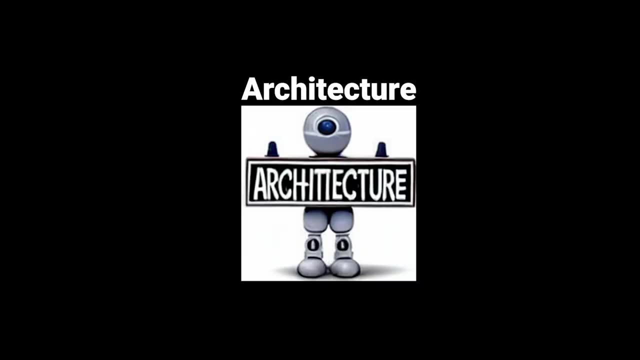 linear schedule Which is too rapid in destroying the information and too uninformative at the end. So we have talked about what the model will take in and predict. Let's take a look at the architecture of it. The authors from the 2020 paper went with a u-net like architecture. 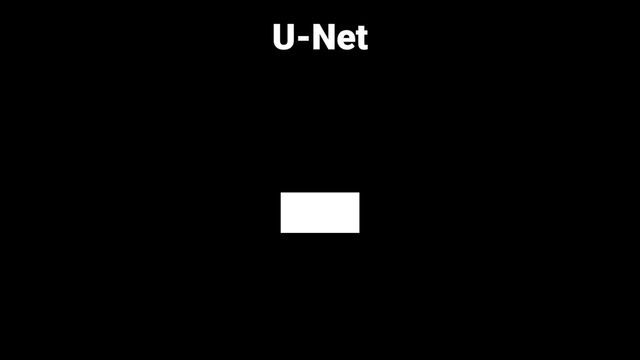 This kind of architecture has a bottleneck in the middle. It takes as input an image and, using downsample and resnet blocks, it projects the image to a small resolution And, after the bottleneck, it projects the image And projects it back up to the original size. 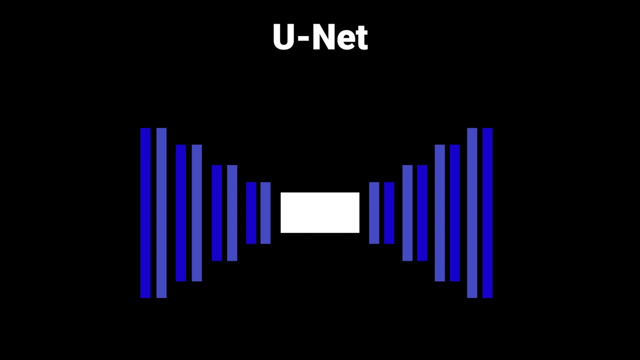 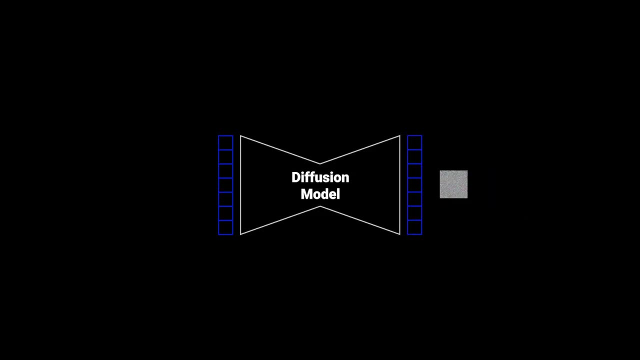 This time using upsample blocks instead, And also at certain resolutions, the authors put in attention blocks and employed skip connections between layers of the same spatial resolutions. The model will always be the same for each time step, And the way of telling the model at which time step we are is done using the sinusodial. 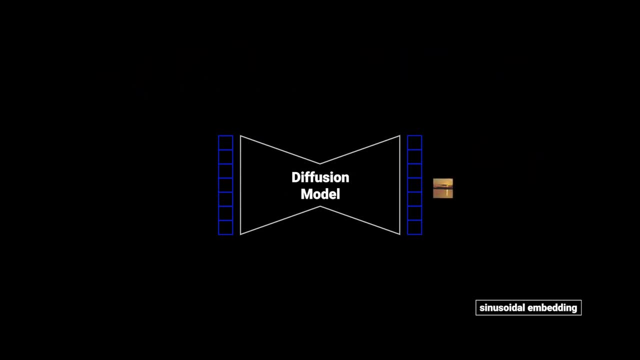 embeddings from the transformer paper. This embedding is projected into each residual block. This is important because the forward diffusion process is using a schedule, as I mentioned earlier, Which scales the mean and the variance. As a result, different amount of noise is applied at different time steps. 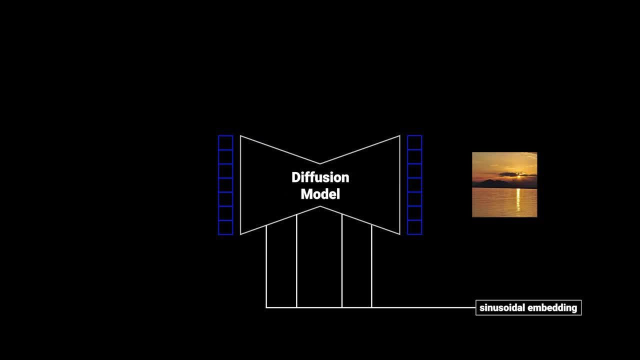 And with this information, the model can also take care of removing different amount of noise at different time steps, Which greatly benefits the outcome. I will be talking more about the schedules later in the maths part In the second paper from OpenAI. they heavily improved the overall outcome by improving 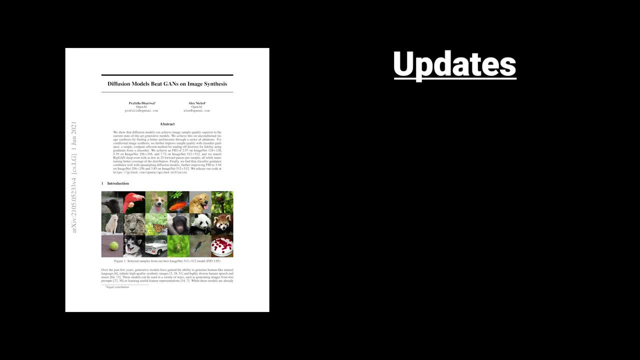 the architecture. They made the following updates. First of all, they increased the depth of the network and decreased the width. Then they included more attention to the size, Then the original proposal, and also increased the number of attention heads. They also took the residual blocks from BigGAN and used this for the upsampling and the downsampling. 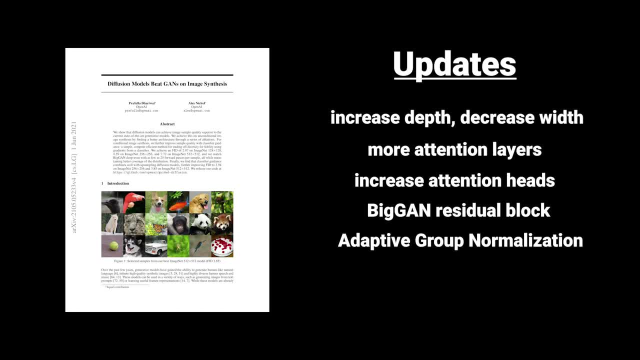 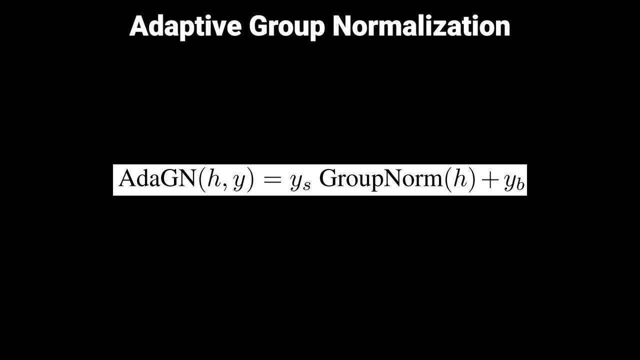 blocks. Next they propose what they call adaptive group normalization. This is just a fancy name for the idea of incorporating the time step- slightly different- and additionally also the class of the label. They first apply a group norm after the first convolution in each ResNet block. 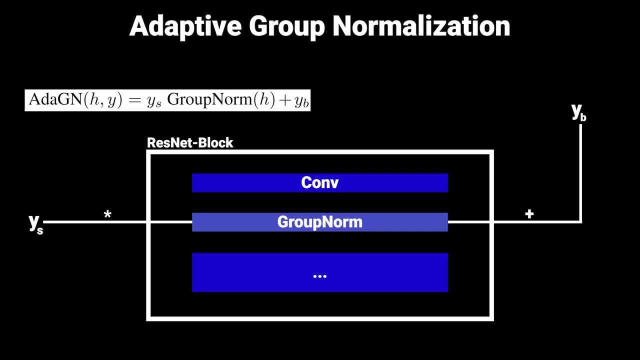 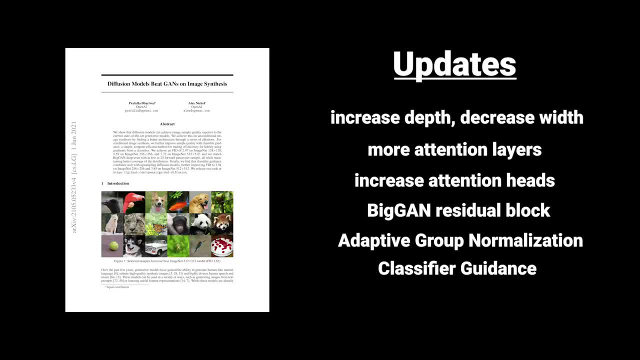 And multiply this by a linear projection of the time step and add a linear projection of the class label onto it. The last improvement is classifier guidance, which uses a separate classifier to help the diffusion model to generate a certain class. However, this is an entire topic on its own and I plan on talking more about this in another. 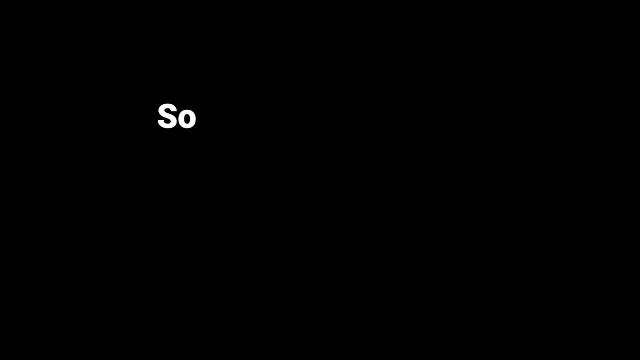 video, So I will not be going into it much in this one. So now you should have a basic understanding of how diffusion models work. To briefly summarize, We have two processes: One for going from a normal image to complete noise which follows a normal distribution. 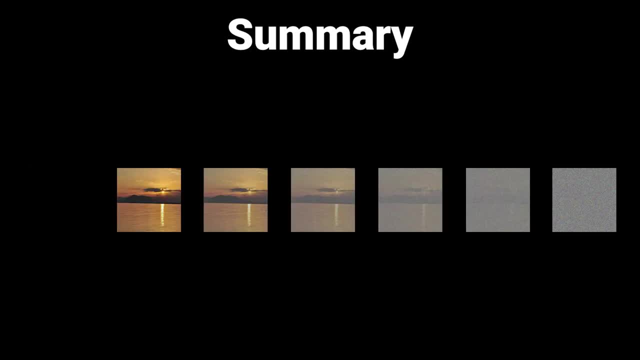 And we have a reverse process, going from complete noise to a real looking image using a neural network. Both processes are done iteratively and the architecture of the model follows a U-Net. Great, now it is time for jumping into the math part, to deeply ground this rough intuition. 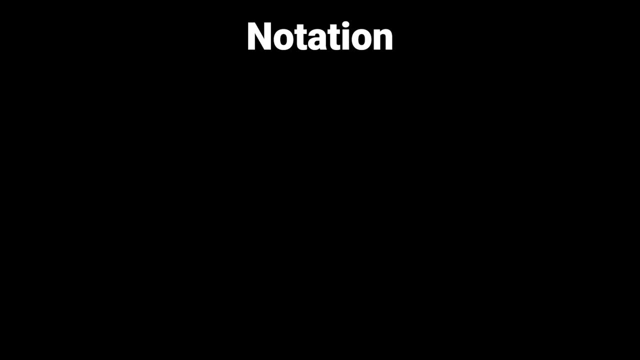 Ok, so let's approach this really easy and start with some basic notation. so we are all on the same level. We will define our image as x, with a number as a subscript. This number will determine at which time step we are. So x0 will refer to the original image and as time passes and we add more and more noise, 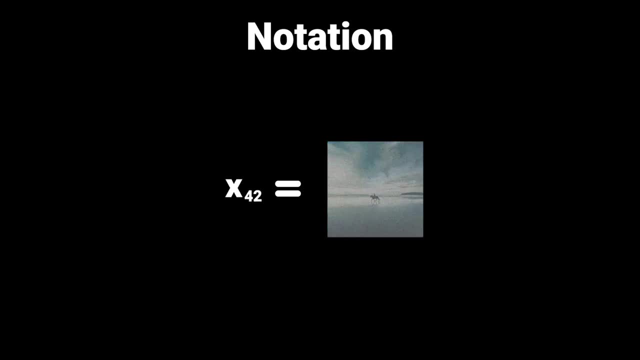 this number will increase. For example, x, subscript 42 will be our image. after applying 42 iterations of noise, The final image, which follows an isotropic Gaussian, will be called x. T also varied throughout the papers. Initially it was set to 1000. 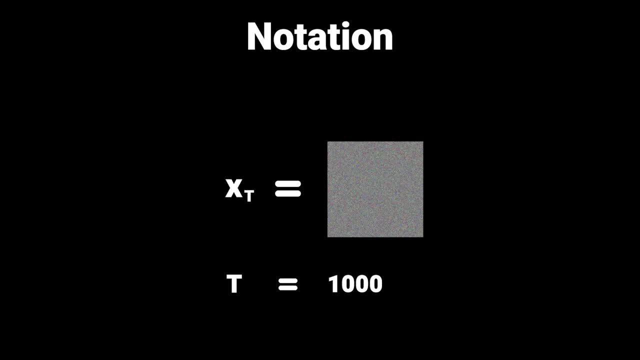 However, the follow up papers were able to decrease this number to just a fraction. Next up, we will define two functions, Q of xt, given. xt-1 corresponds to the forward process and takes in an image and returns an image with a little bit more noise added. 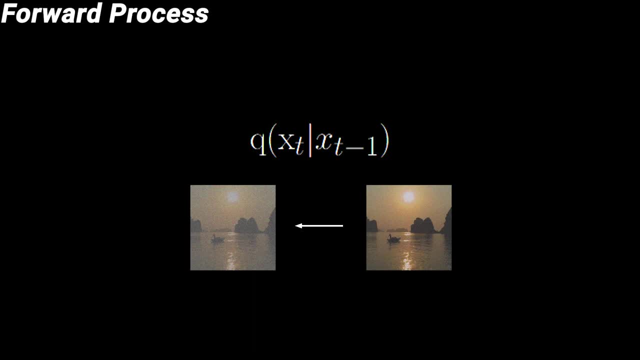 So xt-1 goes in and out comes xt, which has more noise. We will be using this notation often and, in order to not get confused, you can remember that t-1 always corresponds to a less noised image and, on the other hand, t corresponds. 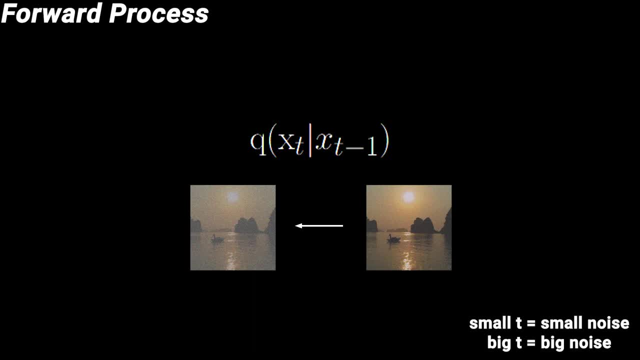 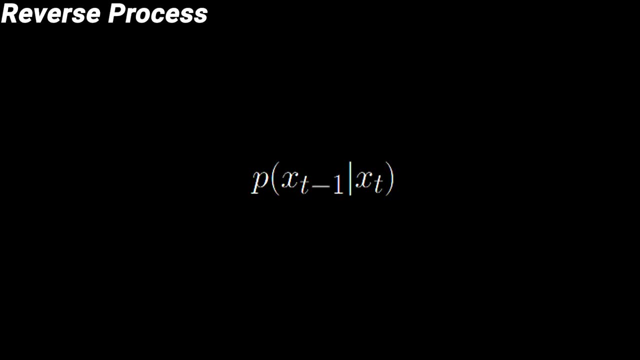 to an image with more noise. In short, a smaller number means a smaller number. In short, a smaller number means a smaller number And a bigger number means a bigger amount of noise. The second function is for the reverse process, and we will call it p. 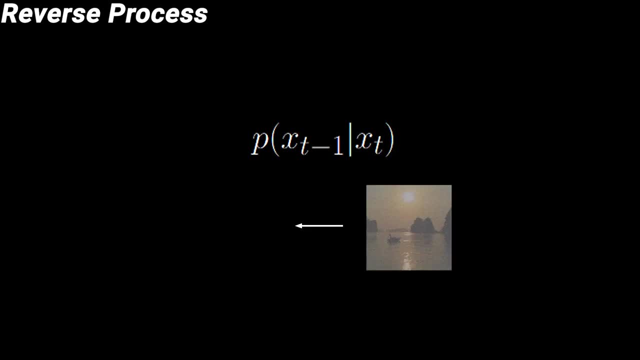 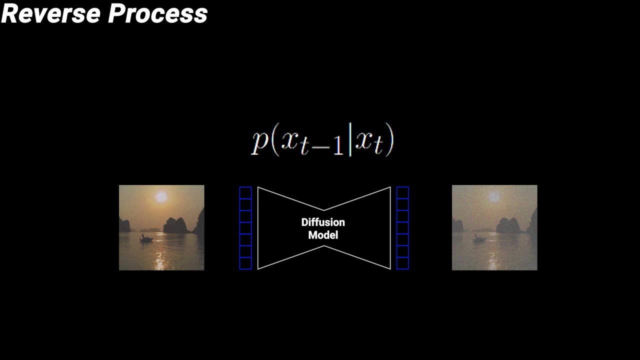 p takes in an image xt and produces a sample xt-1 using the neural network. So this time xt goes in, which, if you remember from before, has more noise, and out comes xt-1 with less noise. Great, and with this knowledge we can now dive into the forward process. 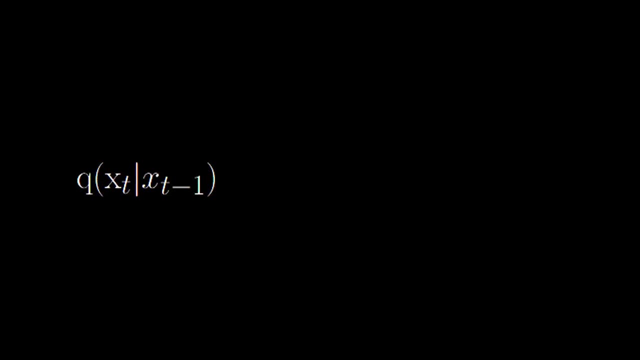 So Q of xt, given xt-1, will be defined as xt-1.. We will be using this notation for the forward process And, don't be afraid, by this formula it is fairly simple, just the notation is a bit frightening. Let me explain. 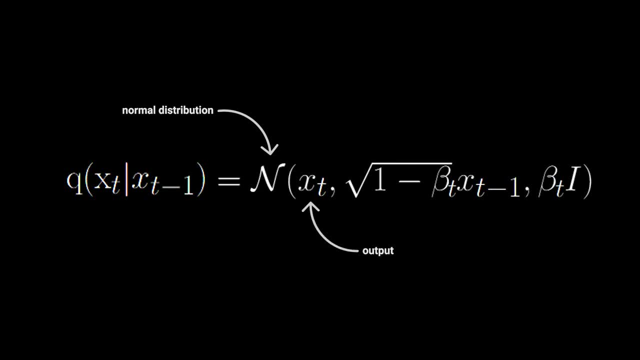 n is the normal distribution, x of t will be the output. this term will be the mean and this term will be the variance. Beta refers to the schedule I was talking about before. All betas will be ranging between 0 and 1 and are ensuring that the data is being scaled. 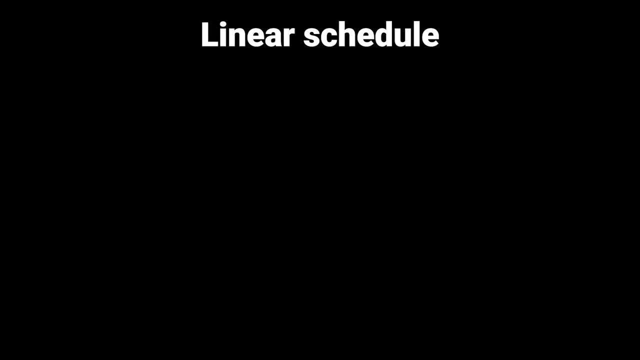 so that the variance doesn't explode. To better understand this, let's take a closer look at the linear scale. Let's take a closer look at the linear scale. Let's take a closer look at the linear scale. They defined the smallest beta to be 0.001 and to grow linearly up to 0.02.. 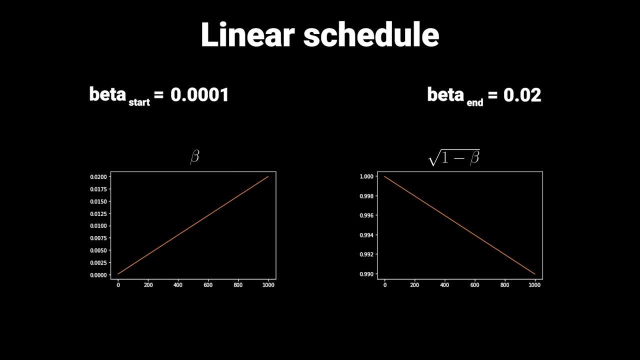 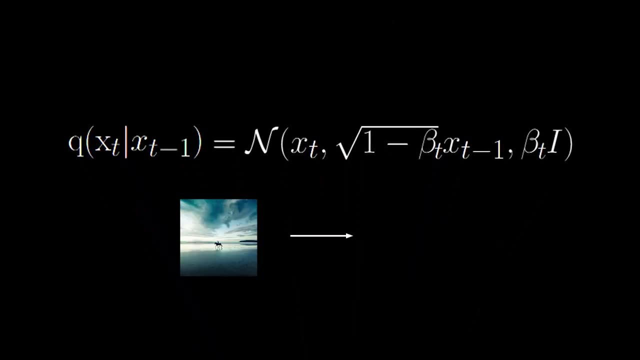 Plotting both beta and the square root of 1-beta against time results in the following two plots: You can see that we more and more scale down the image which acts as a counterpart for increasing the variance over time and keeping the variance inbound. We now understand how to apply one forward step. 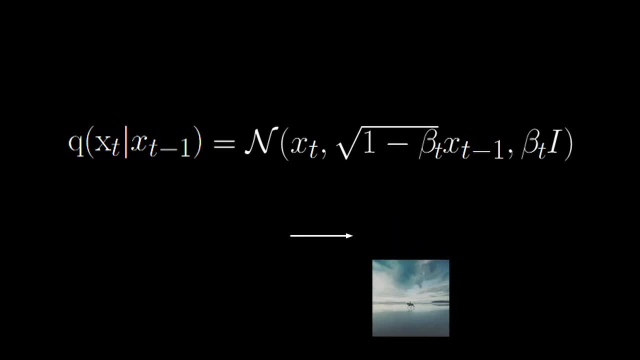 To apply, say, 1000 forward steps. We could easily repeat this formula a thousand times, But there is an easier way of doing this in just one step. How cool is that? For that we need to define a little more notation. So, bear with me, it's not much. 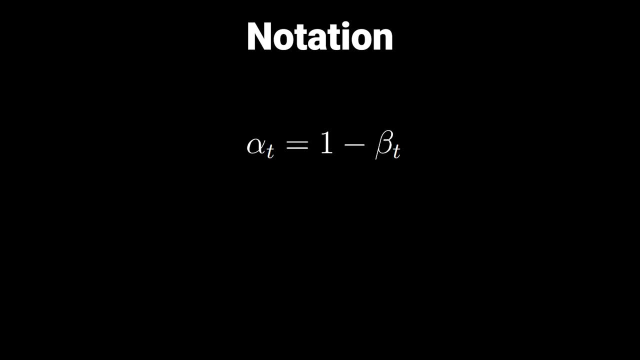 We'll define alpha t to be 1-beta t and then we'll also define the cumulative product of all alphas from 0 until t. So we just multiply all alphas together. You'll see in a second how we are going to use this. 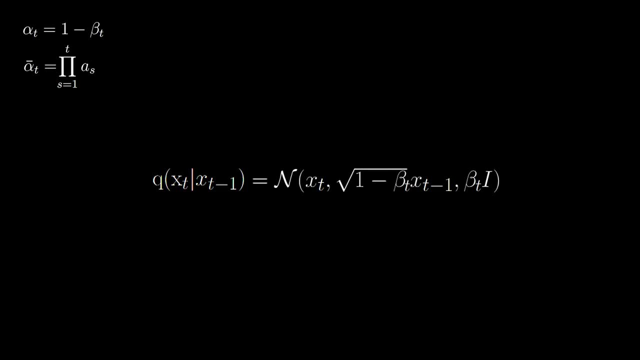 Alright, First of all, We need a more established formula for one time step like the following: using the re-parameterization trick, Epsilon is taken from a normal distribution with mean 0 and standard deviation of 1.. Now we rewrite it using alpha. 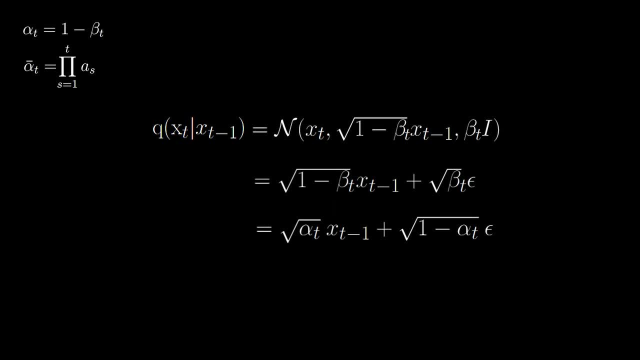 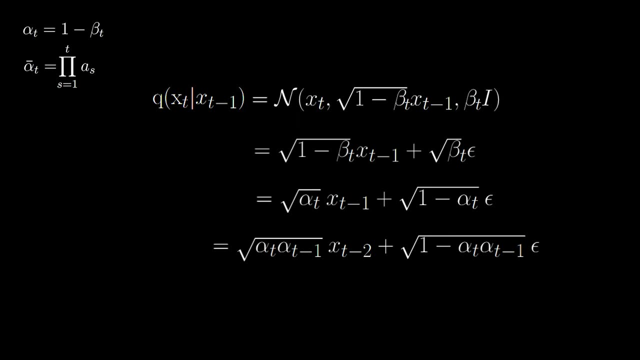 Pause the video to see that they are actually equal. And now comes the trick. We can extend this to earlier time steps and go from t-2 directly to t by just chaining the alphas, And also from t-3 to t, and so on. 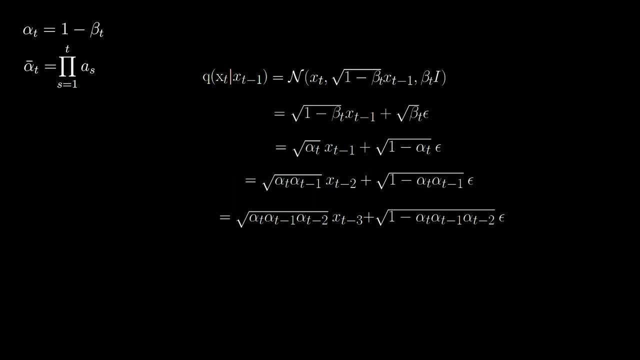 And you see where this is going. We can go all the way to the beginning and go in an instant fashion from x0 to xt. And now you also understand why we introduced the cumulative alphas: To simply shorten the formula. All of this can now be also rewritten in the original form, like this: 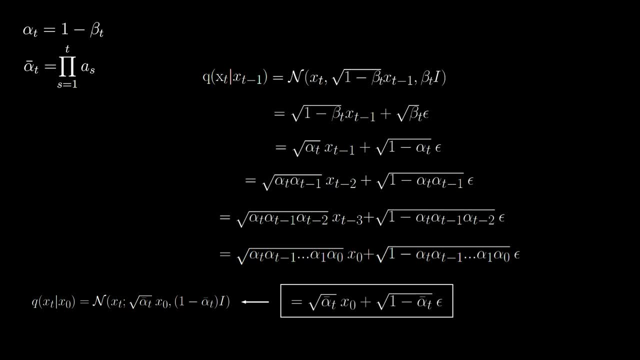 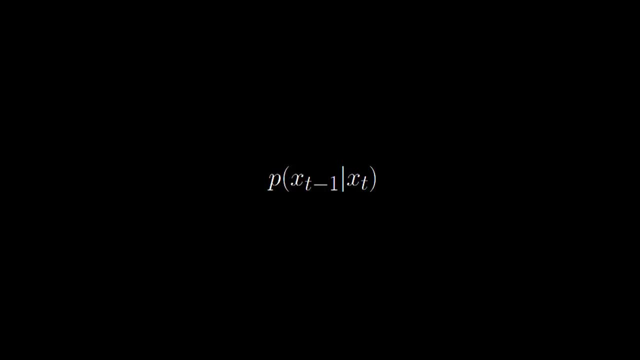 And that's already it for the forward diffusion process. It isn't that hard right. So now let's move to the reverse diffusion process. So, if you remember, we already established the notation for the reverse process and called it p. We can also express this formula in the following way: 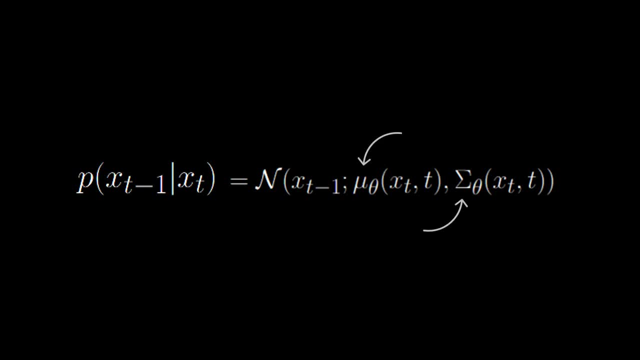 In that case we would have two neural networks which parametrize the normal distribution which we can sample from to get xt-1.. We already said that we fixed the variance to a certain schedule, so we don't need to predict it and can take this as given. 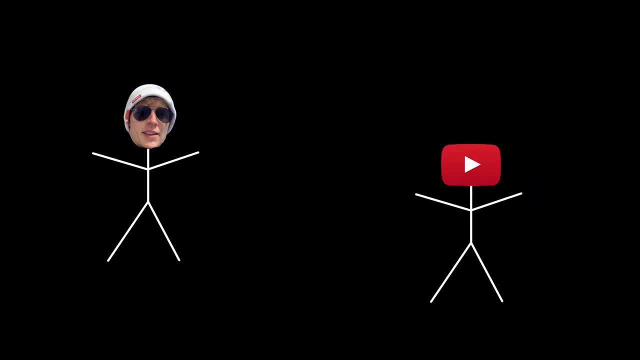 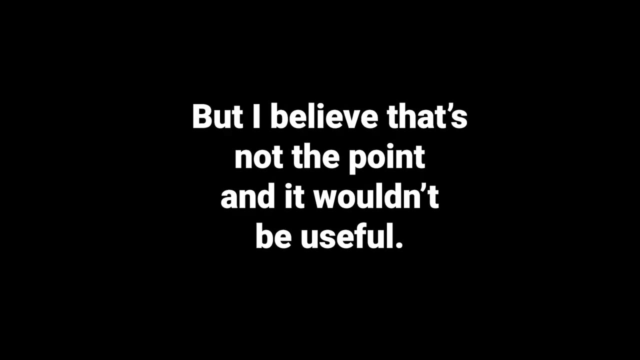 Now I could just throw you the rest of the formulas at your head and say that you should take this for granted. Then the video could be over in less than a minute. But I believe that's not the point And it wouldn't be useful. 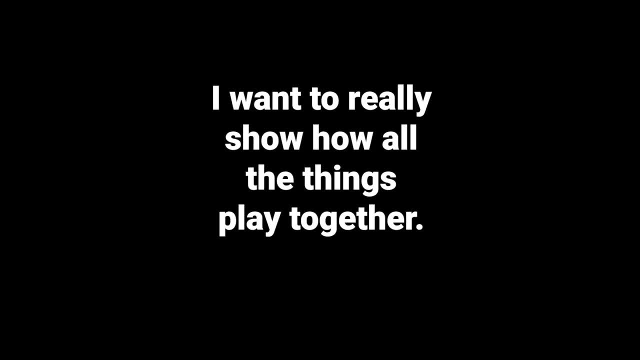 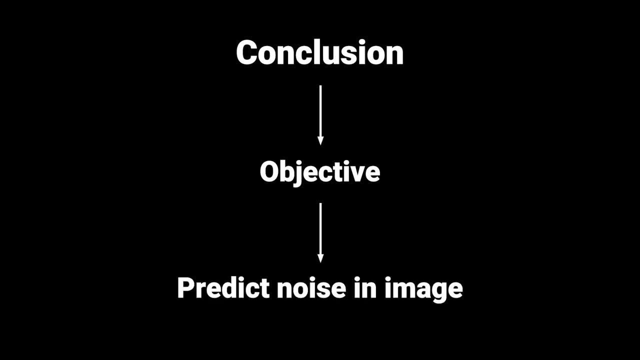 As a result, I want to really show how all the things play together to come to the conclusion which leads to the final objective where we just have to predict the noise. So that's the end goal: Arriving at a formula which uses a neural network to predict the noise in an image between 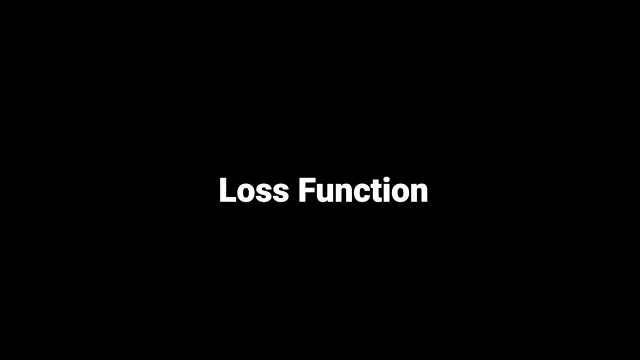 two time steps. Keep that in mind. In order to have the easiest time, we will start by looking at the loss function of this whole thing. This will simply be the negative log likelihood. But there's a problem. The probability of x0 isn't nicely computable as it depends on how much time we have left. 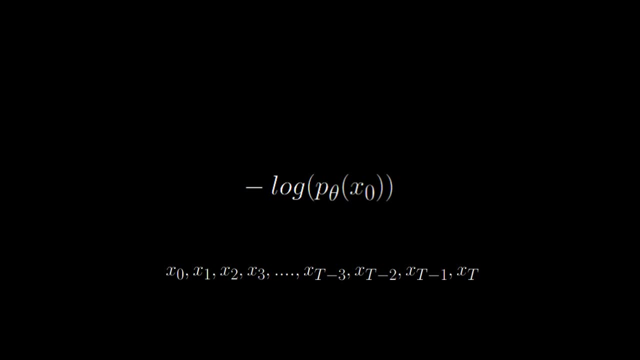 It depends on all other time steps coming before x0. Starting at xt, This would mean keeping track of t-1 other random variables, which is just not possible in practice. As a solution, we can compute the variational lower bound for this objective and arrive. 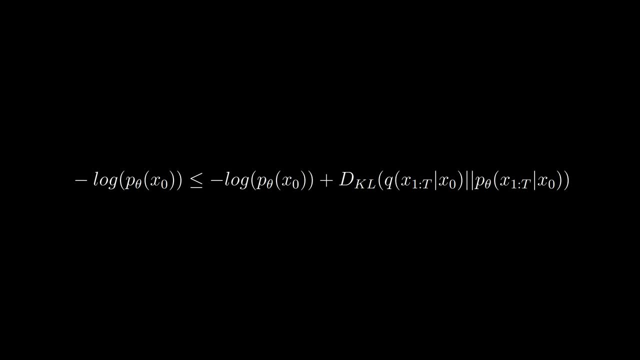 at a more nicely computable formula. Note that the overall setup of diffusion models is pretty similar to that of variational autoencoders, So make sure to look that up if some of the things may be unclear to you. I also put some references in the description. 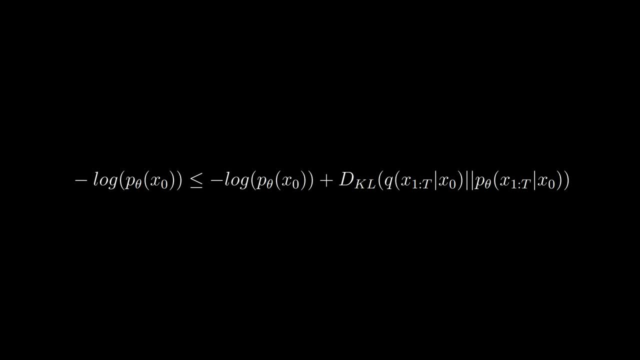 If you're not familiar with the idea of a lower bound, let me give you some intuition. Say we have some function f which we can't compute- In our case the plain negative log likelihood- And we can prove that we have some function g which is always smaller than f, which 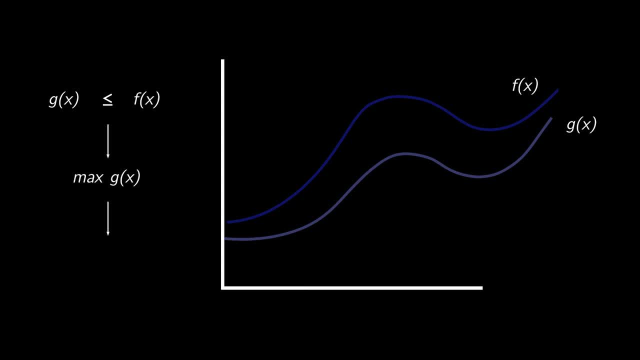 we can compute. Then by maximizing g, we can be certain that f will also increase. In our case, this would be ensured by subtracting the KL divergence, which is a measure of how similar two distributions are, And is always non-negative. So by always subtracting something non-negative from a function will always result in having 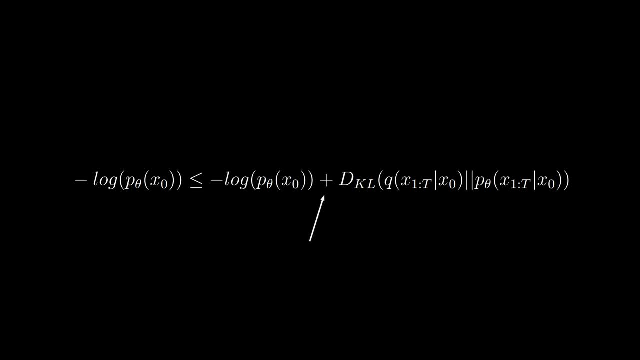 something which is less than the original function, But I wrote a plus sign instead of minus. This is simply because we always want to minimize instead of maximizing. That's why we add it and thus have something which is always bigger than the plain negative log likelihood. 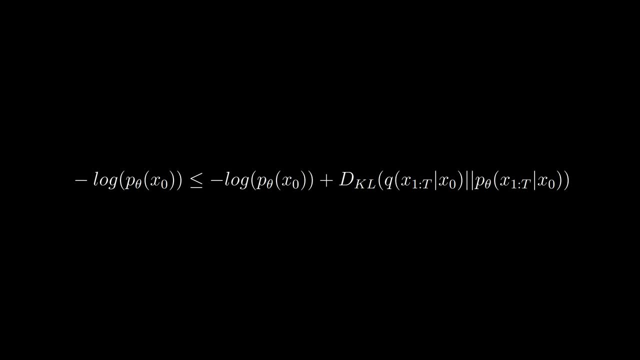 And then we can minimize this objective. However, in this form, the lower bound is not computable either, since, yeah, we still have the quantity which we can't compute, And that's why we need some clever reformulations to arrive at a nicer looking quantity. 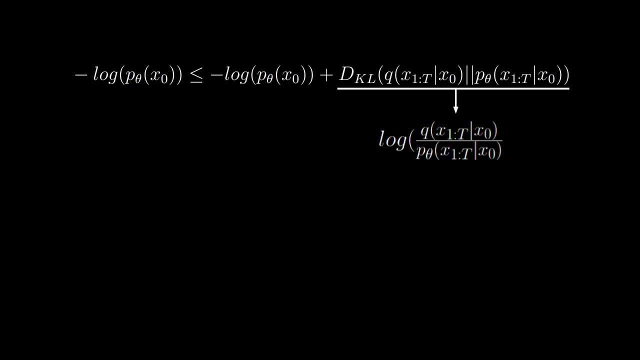 At first we rewrite the KL divergence to be the log ratio between the two terms. Now let's apply the Bayesian rule to the quantity at the bottom. The upper term can be summarized to a joint probability, and now we can see that we can just write this as the probability of x0 until t. 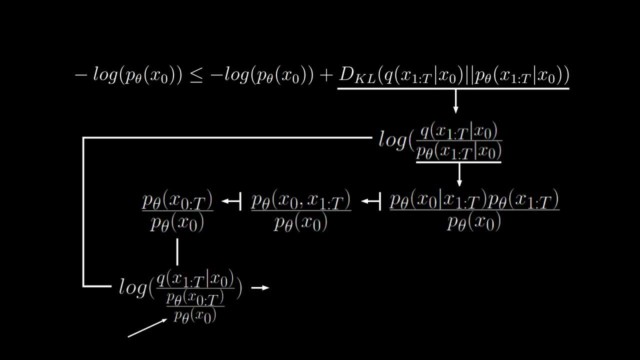 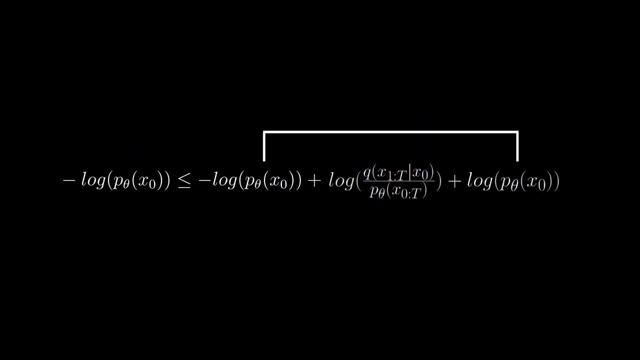 Now we can pull the bottom quantity to the top by using the fraction rules and split up the logarithm, And now you already see the magic: These two terms just cancel each other, and thus we get rid of the annoying quantity which we can't compute. 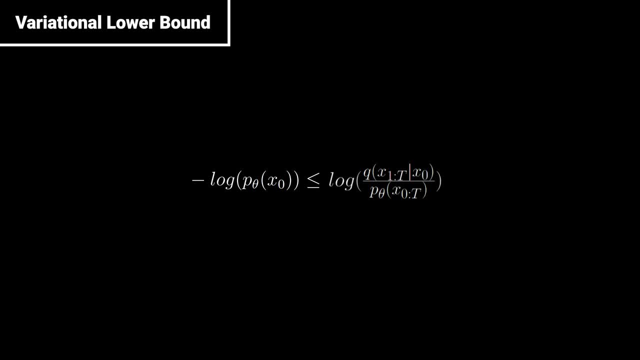 Great, now this is our variational lower bound, which we can minimize, And note that we know all of these things. The term at the top is just a forward process, starting at some image from our data, and the lower part can be rewritten as the following: 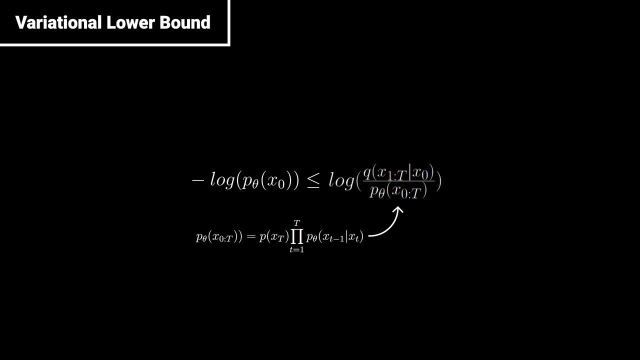 And you see that we can calculate p and the product of all these terms is just using our parameterized model p. Now, in order to make this analytically computable, the authors applied a couple more steps of reformulation to arrive at a nice looking lower bound. 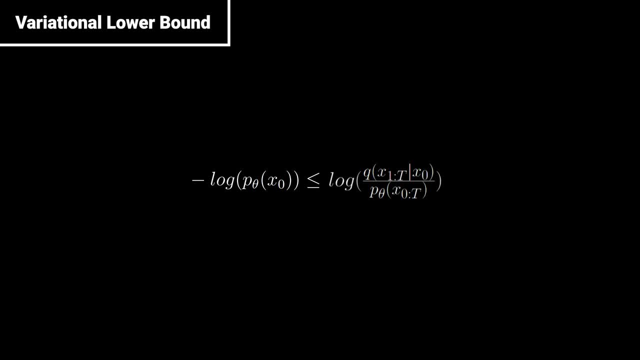 Which we will also do now, And I promise this will be the last math-heavy part. So let's take our current lower bound and write it in product form, which I showed before. By applying the log rules, we can bring out p from the denominator, so that we are left. 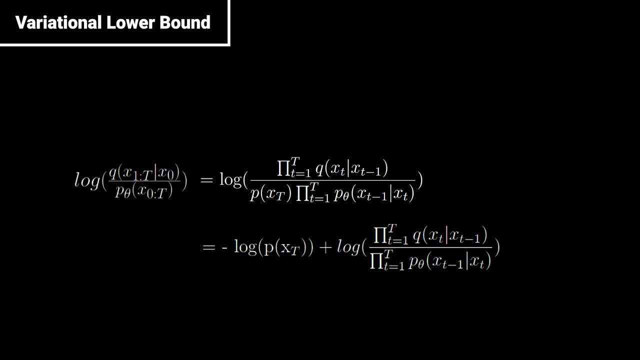 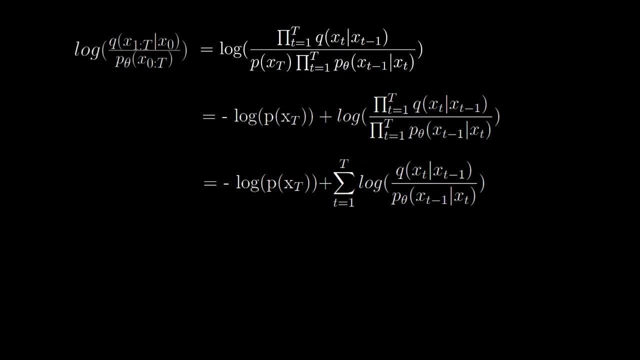 with the fraction of the forward process and the reverse process. Next, we apply more log rules to bring out the product Which becomes x0.. Now the authors do something which might appear weird at first but will make sense in a minute. They take out the first term of the sum, which now starts at t equals 2 instead of t equals. 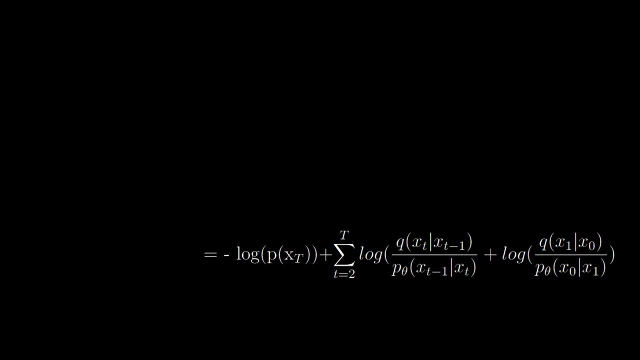 1. So they split up the first term from the entire sum. They now rewrite the denominator in the sum using Bayes rule, which can be expressed like this: Pause the video and see for yourself. It's just a standard Bayes formula. 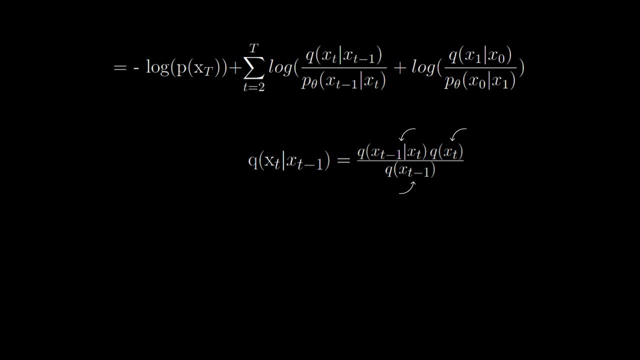 Now there is a problem. All of these quantities have a really high variance, since we don't know what we started from. So this is why the authors drastically reduced this variance by also conditioning on x0. Because just imagine this: Given this picture, you might be pretty uncertain where it came from. 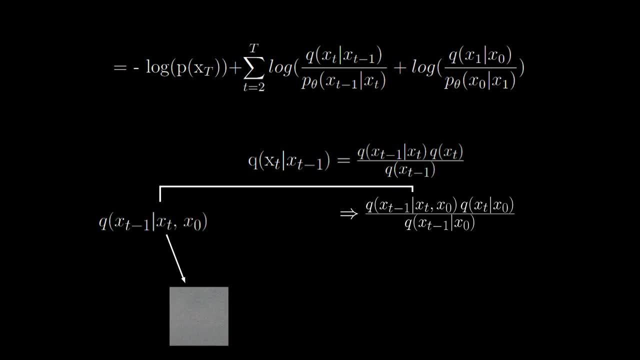 So there's a high variance. But say, I also give you the original noise-free picture. now The choice for possible candidates decreases and you might be more certain And it gets even better. This formula has a closed-form solution which I will talk more about later. 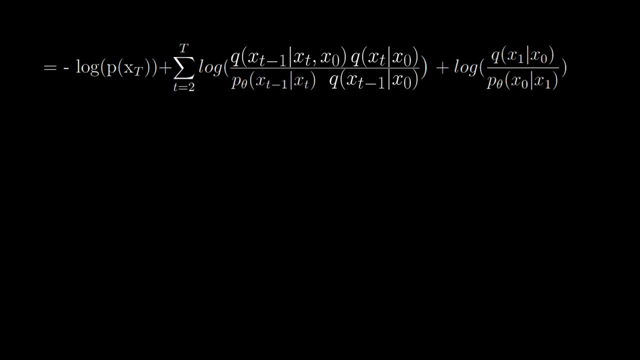 Fusing this back into the formula will give the following, And now you might already see the reason why. I see the reason why we pulled out the first term. If we hadn't done this, the first term would look like the following: after applying Bayes: 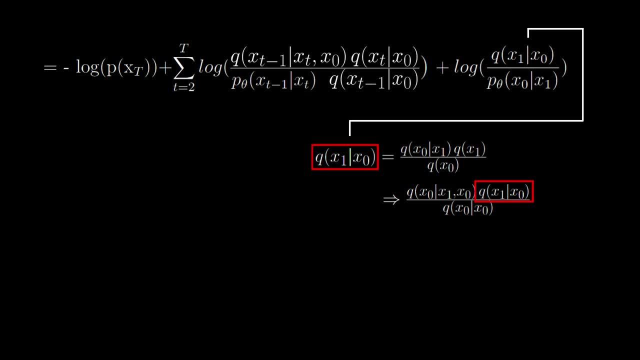 rule and conditioning on x0.. You see that we have a loop and other things which don't really make sense. Ok, now we almost made it, Just a few more modifications to be done, So bear with me. First, we split up the summation in two parts because we can. 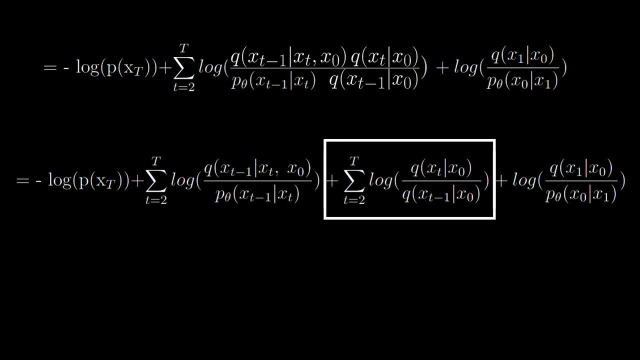 Now let's take a closer look at the second summation. See something? Let's take an example case and say: capital T equals 4.. So we have x0.. So capital T equals 4.. Writing the summation out will give us the following: 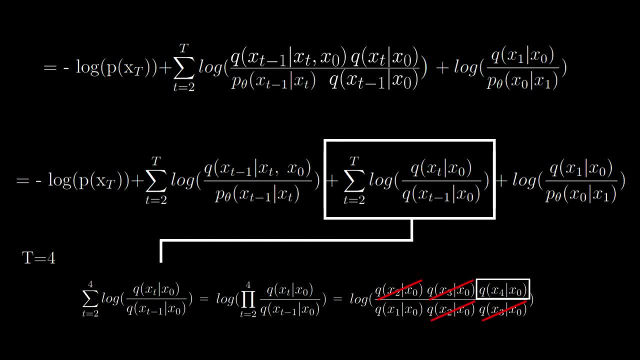 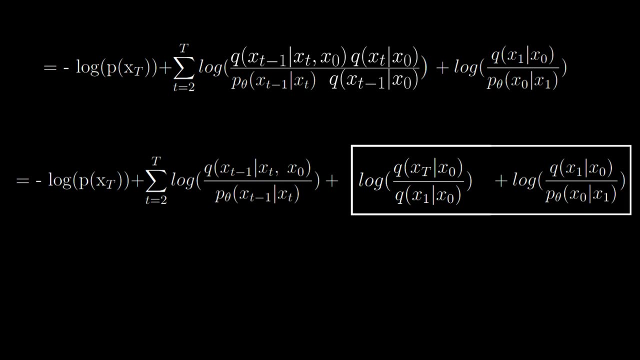 And you see that most of the things cancel and only the last term from the top and the first term from the bottom survive. That's why we generally can simplify the summation to just this, And now the formula will look like the following: Now for the last step. we take a closer look at the last two terms and, by applying the 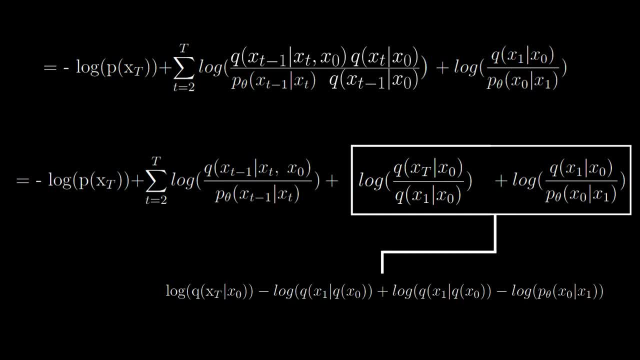 log rules and converting the inner quotient into an outer subtraction, we see that these terms cancel each other. Now the authors bring this term to the front and fuse them in one logarithm, Which leaves us with the final analytically computable objective. We can now write the first terms in KL divergence notation. 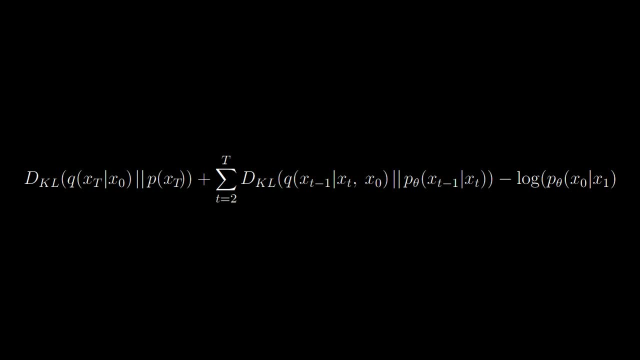 And voila, objective. And it gets even better. We can ignore the first term completely, since Q has no learnable parameters, it's just a forward process which adds noise over and over, and P is just random noise sampled from our Gaussian and also by the aforementioned theory that Q will converge into the first. 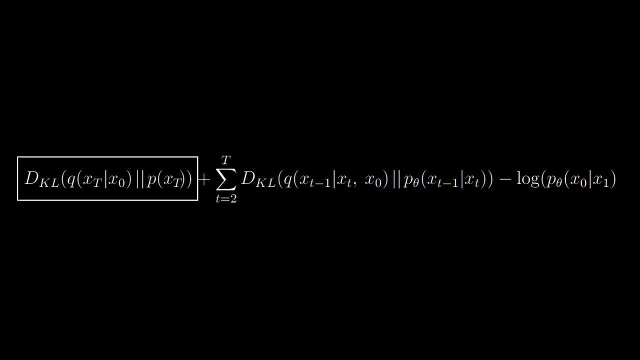 term converge to a normal distribution, we can be certain that the KL divergence will be small. I also want to give one more hint, since often these big math derivations might be logical and one can follow them, but you barely understand why this is being done. 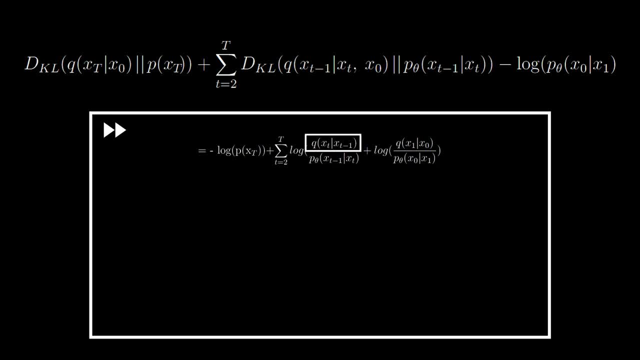 And the most crucial part of the previous derivation is the part where we apply Bayes rule to convert Q given to this equation. Obviously, one can understand that this is true, but it doesn't seem obvious- at least it didn't to me- what the reason for that is. 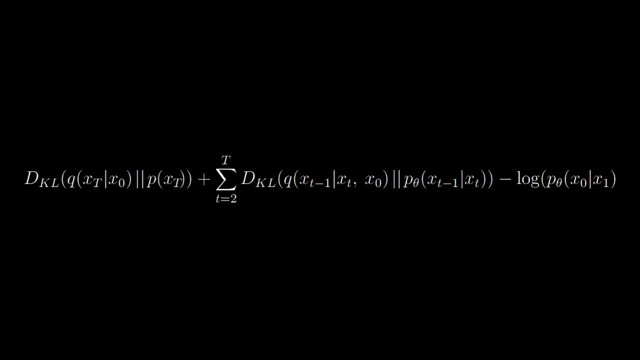 And to give some intuition for the reason, we can take a look at the final objective. Look at the second KL divergence. It is a really nice quantity which we can compute, as we will also see later, And deriving at this would have not been possible if we hadn't applied Bayes rule. 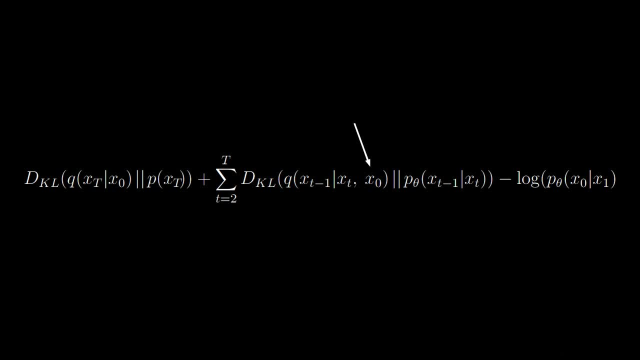 This reformulation and the extra conditioning on X0 gave us the possibility to have the forward process in the same form as the reverse process, And we also saw the other additional benefits where a lot of things cancelled or simplified. So we are left with these two terms. let's first focus on this one. 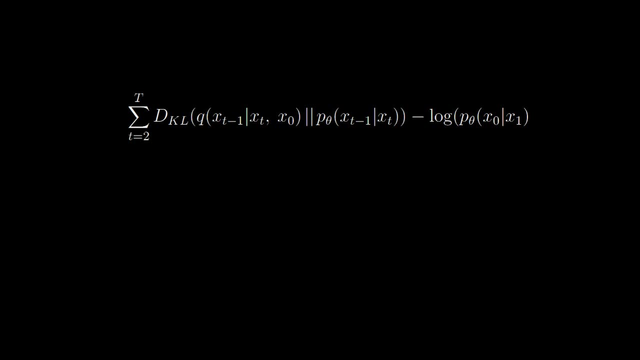 We already showed that we can express P given Xt like this. Nothing new here. One new network for the mean and one for the variance. however, the variance is a fixed schedule, as discussed before, And I also mentioned that Q given Xt and X0 has a closed form solution which we can. 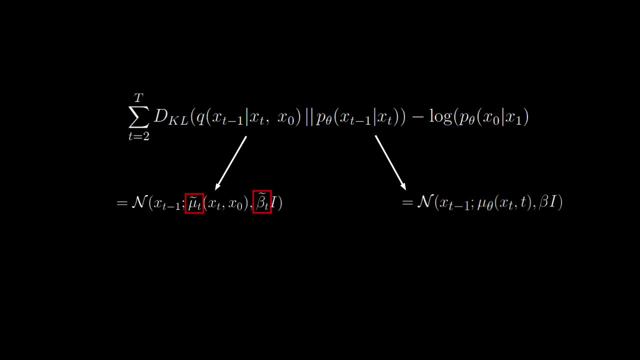 also write in the form, like we did with P Deriving mu and beta would take quite a bit of time and would make the video even more interesting. So we are left with these two terms. let's first focus on this one. We already showed that we can express P given Xt like this: 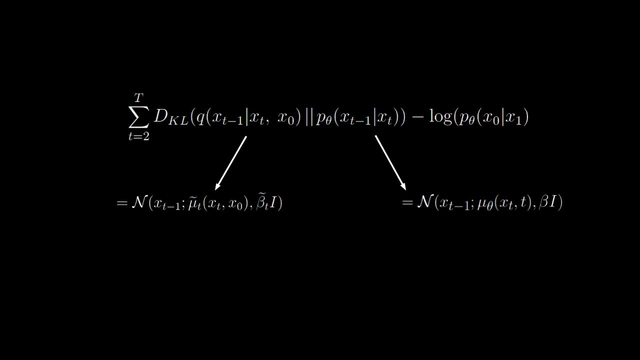 Nothing new here. We already showed that we can express P, given X0 has a closed form solution which we can also write in the form, like we did with P Deriving mu, and beta will take quite a bit of time and would make the video even more interesting. 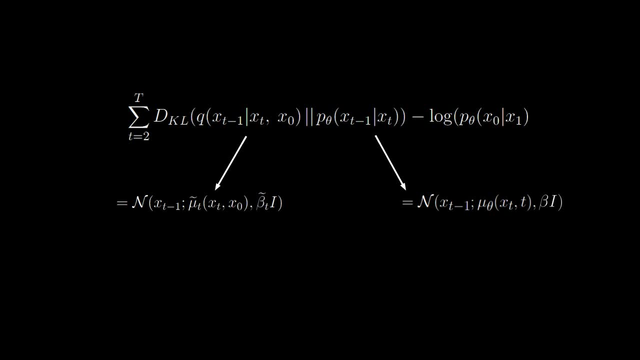 That's why I decided not to do this derivation here, since it is also not relevant for understanding the algorithm. However, I will put a link in the description where you can find more about it. So the final version for mu and beta will look like this: 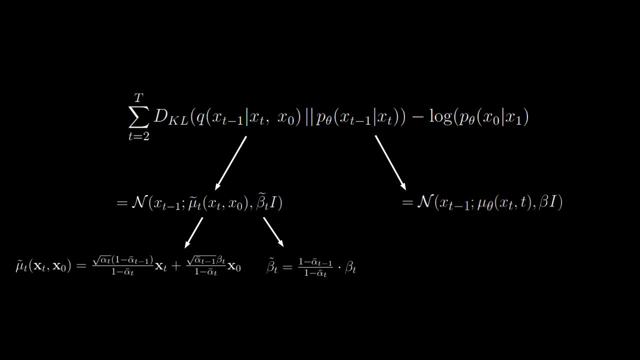 Big formula, I know, don't be afraid, we'll get rid of it Again. beta is not relevant since it's fixed, so let's focus on mu. We can simplify this formula. How Remember the closed form of the forward process for generating Xt in one single step? 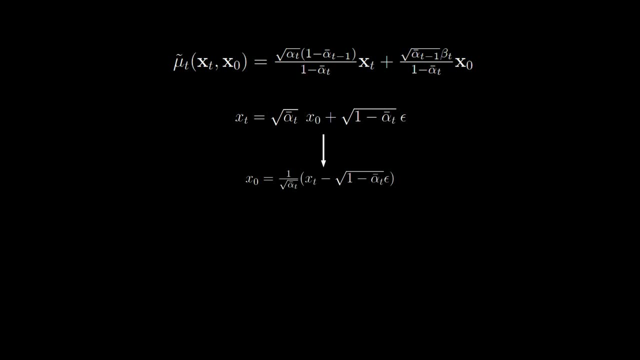 We can rewrite this in terms of X0 and express it like this: Plugging this into mu of Xt and X0 will give us this, And you also see that mu doesn't depend on X0 anymore, And through some further simplifications we end up at this tiny formula. 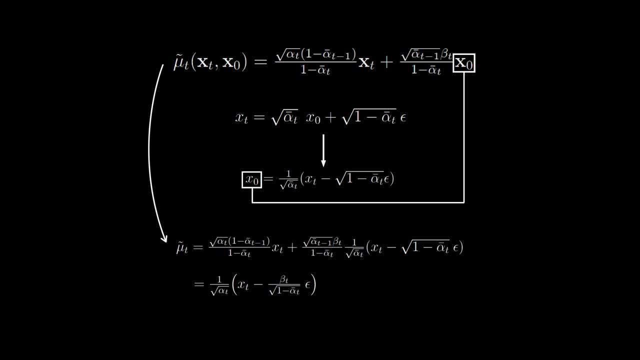 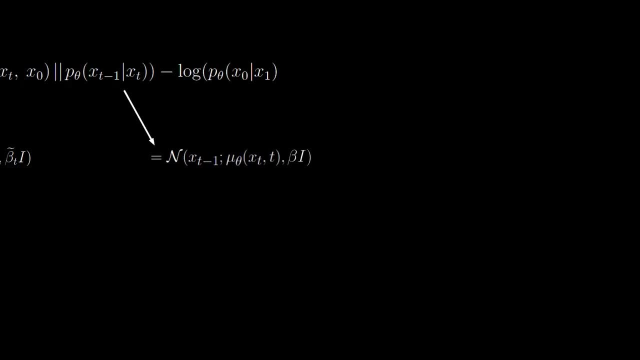 And you see that essentially, we are just subtracting random scaled noise from Xt. That's it And again. take a look in the video description to see the full derivation. Now, this is what our neural network mu needs to predict, and the authors decided to use. 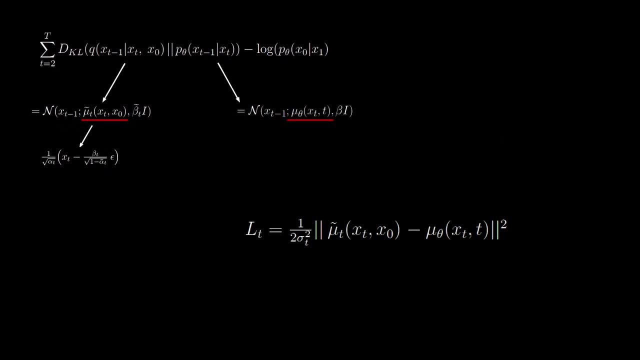 a simple mean squared error between the actual mu and the predicted mu. And now they saw the following: Xt is available as input to the model, So why predict this whole quantity and not instead just the noise? And that is why we can rewrite mu like the following: 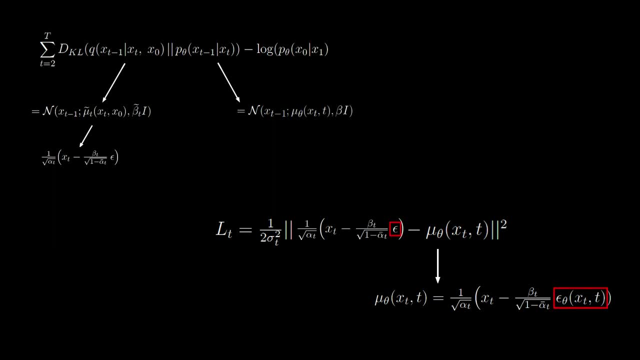 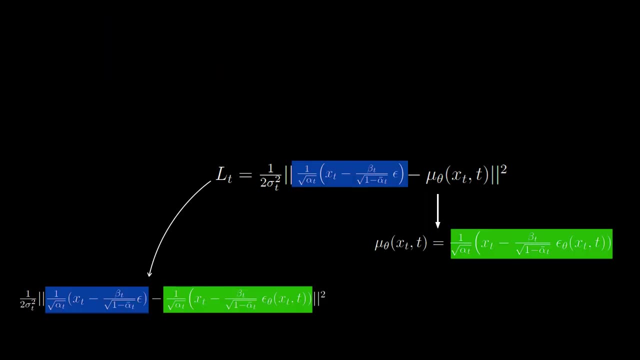 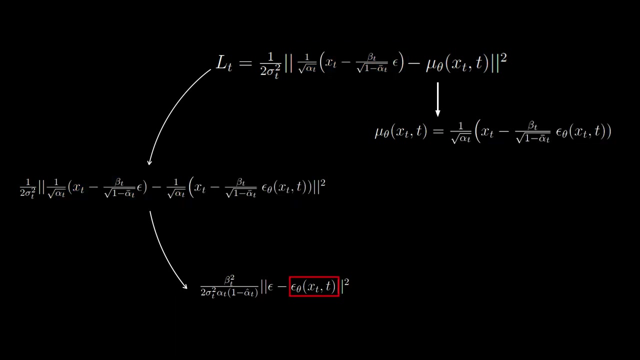 And, as you see, it's completely the same as mu, except for epsilon which is supposed to predict the noise. So let's rewrite the mean squared error like this And through simplification we arrive at this friendly quantity: Just the mean squared error between the actual noise at time t and the predicted noise at. 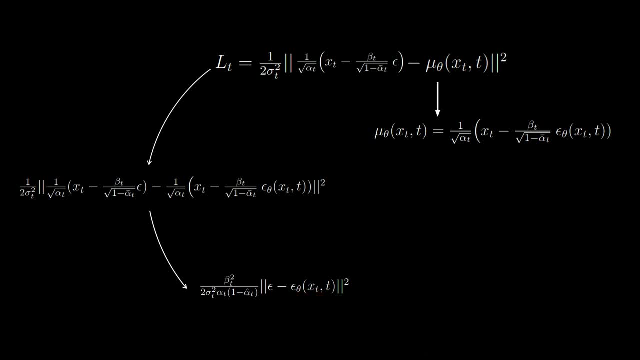 time t by our neural network given some image And, believe me or not, this quantity is about to become even more friendly. The authors found that ignoring the scaling term at the front results in better sampling quality and generally an easier implementation. And I mean, look at this, all of this heavy math derivation, starting at the negative. 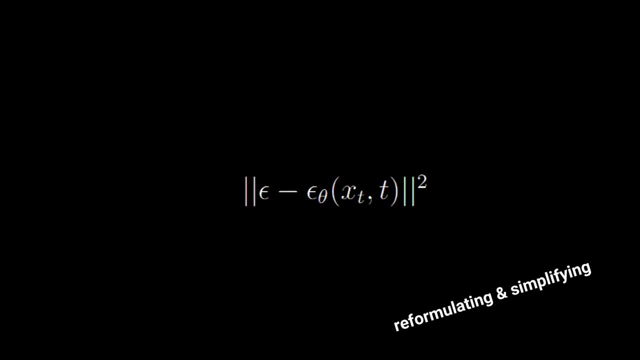 log likelihood, going to the lower bound, reformulating and simplifying this lower bound, seeing that we only need to predict mu, We only need to predict the mean, which leads us to the insight that we only need to predict the noise, and then simplifying even more, because it just works better. 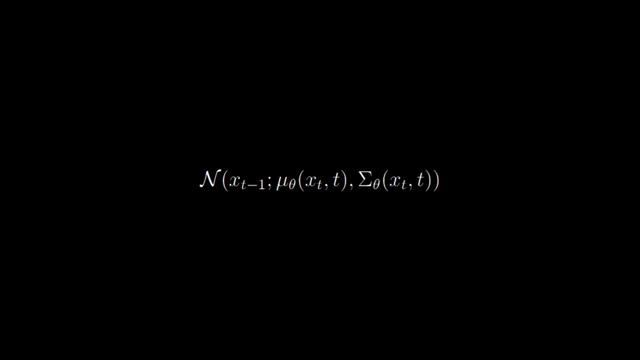 Isn't that beautiful. So, getting back to our starting formula, we can now put in our new findings. The neural network for mu becomes this and once again, the neural network for the variance is not needed and can be replaced by beta t. And to actually sample Xt-1, we can apply the reparameterization trick again and arrive. 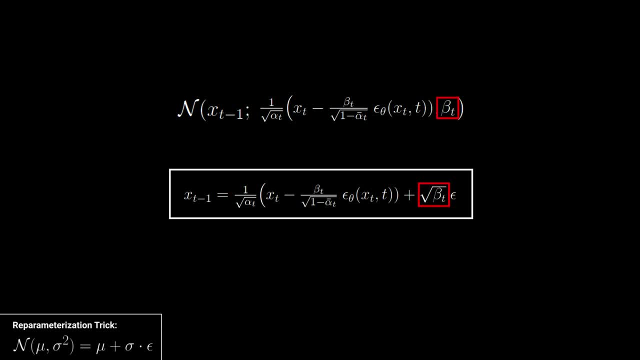 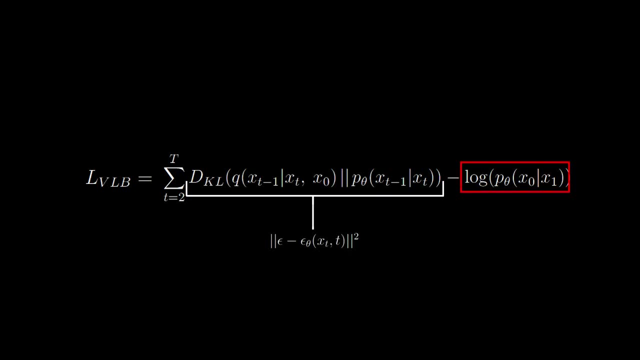 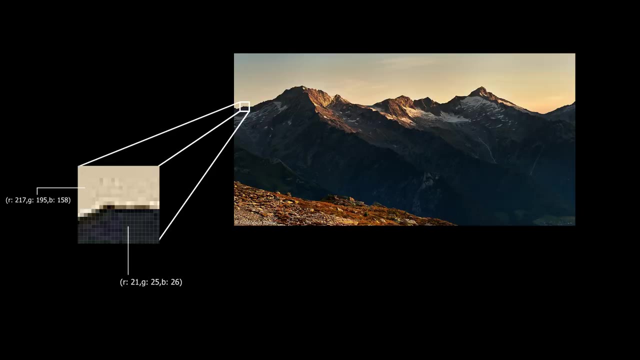 at this equation, We can now get the result of the equation, which is the same as the equation for mu, plus the standard deviation, plus noise sample from a standard normal. Now there's one more thing which we haven't talked about yet. The last term in our lower bound also needs to be taken care of. 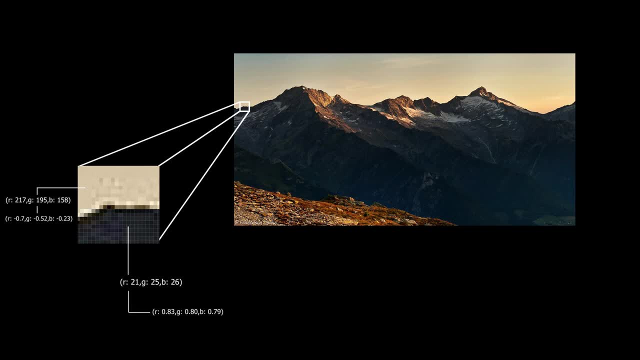 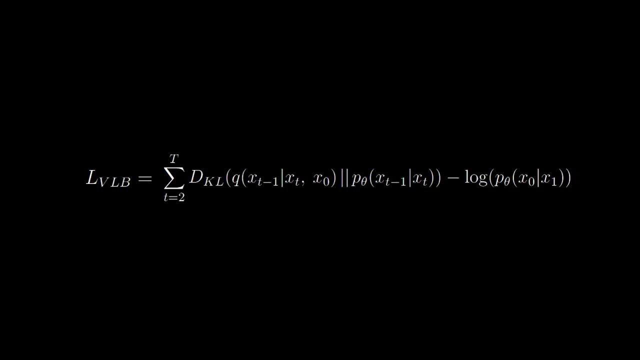 For up some clarification. Images have values between 0 and 255.. The authors scale the images to be between minus 1 and 1 to have them in the same range as the prior standard normal distribution centered at 0 with variance of 1.. 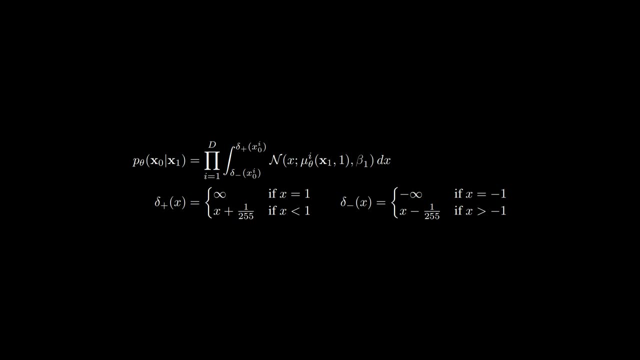 So if we take a look at this- Ok, that was maybe a bit too much at once, but stay with me, I'll explain- D is the data dimensionality, which is the number of all pixels in our case. So we iterate over all pixels in the image. 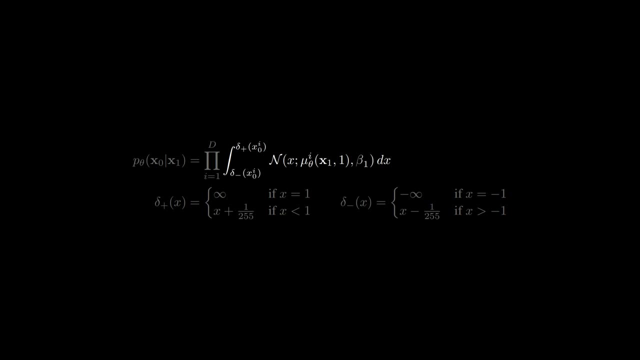 Then we have this evil looking integral. but this just means that we integrate over the range around the actual value of the pixel in X0. And if this quantity actually predicts a mean value in the area of the true pixel, then the integral will be high. 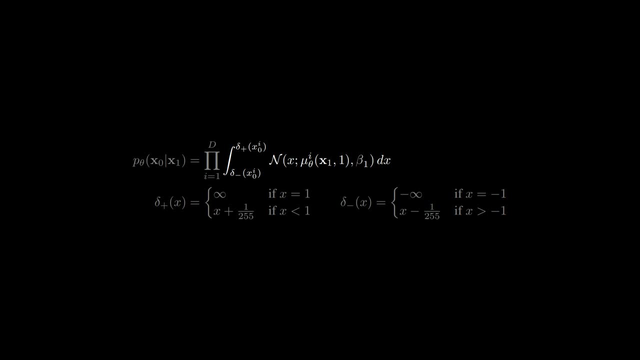 And if that happens for each pixel, then the product will result in a high number and thus the probability of X0, given X1, is high. However, if we always predict a different pixel far away from the true value, then the mass in the true pixel area is low and the overall probability will also be low. 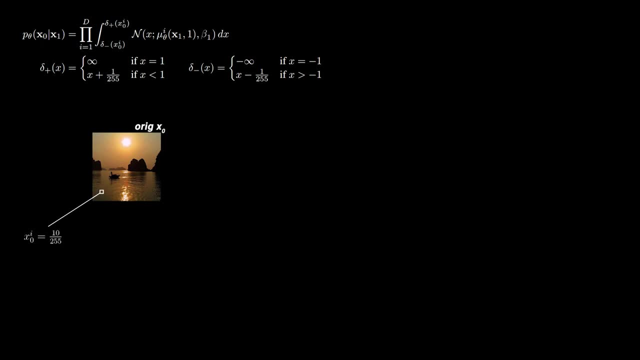 Let's take an example for one pixel. Say the true pixel value would be 10 over 255.. Also, say X1 has a value of 14 over 255 at that specific position We now apply our network and it predicts a new mean of 11 over 255. 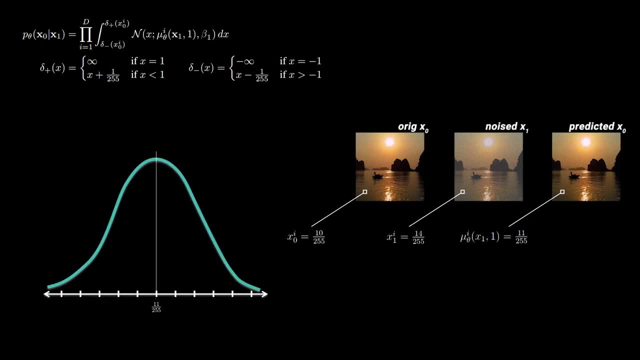 Now we can plot this normal distribution centered at 11 over 255, with some arbitrary variance given by our schedule. And now we could integrate over the true region where the pixel in X0 is starting one pixel value below and going one pixel value above. 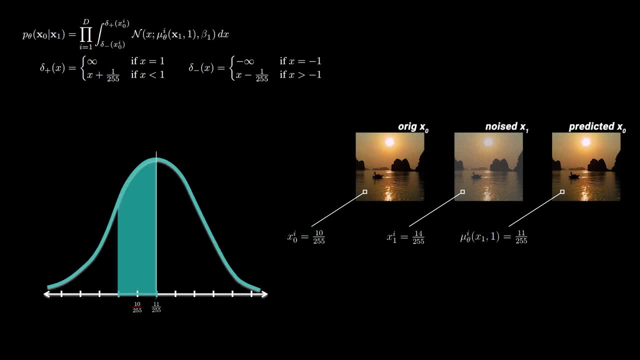 Since the network did a good job at prediction, the mass in that area is quite high. If, however, the network would have predicted a mean of 20 over 255, then we would have the mass in that area would have been super low, leading to a low probability. 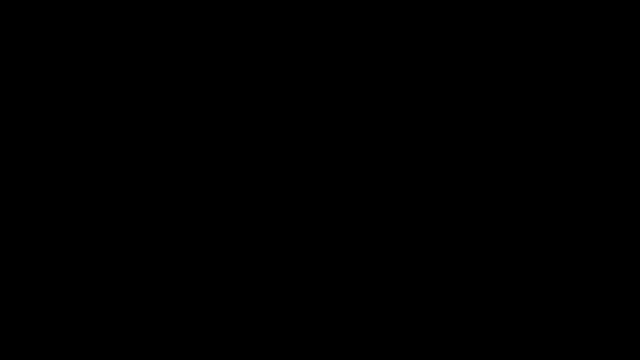 I hope this gives some intuition for understanding the formula. if not, don't worry. the authors also just decided to get rid of it and approximate it by our neural network, and the only difference is that at sampling time we don't add noise to it. 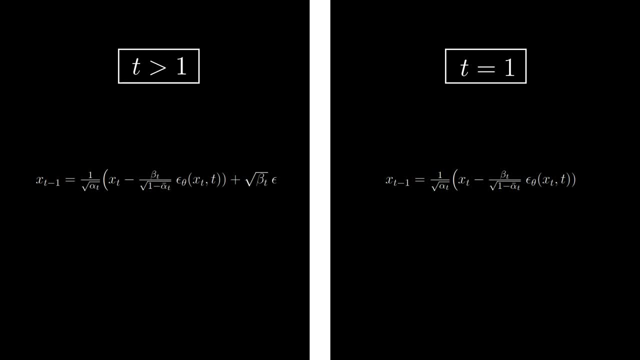 Yeah, that's it. sorry if you just spent your valuable time trying to understand this And now our entire objective fits into one single line and can be written like this: That is what we optimize. T is sampled from a uniform distribution between 1 and T and this long formula in our neural 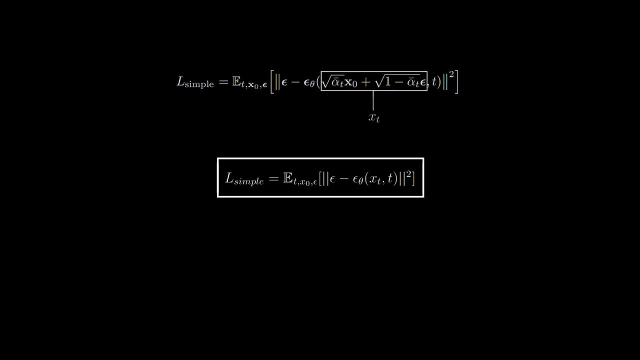 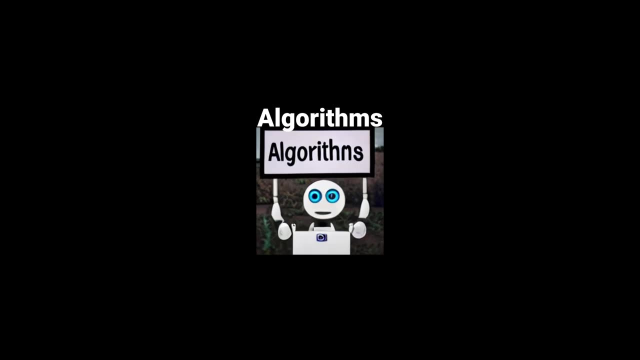 network is just XT, and we could also write it like this. That looks even more peaceful if you imagine where we started. So now let's take a look at the algorithms for training and sampling. summarized, This one is the algorithm for training and you see, we first sample some image from our 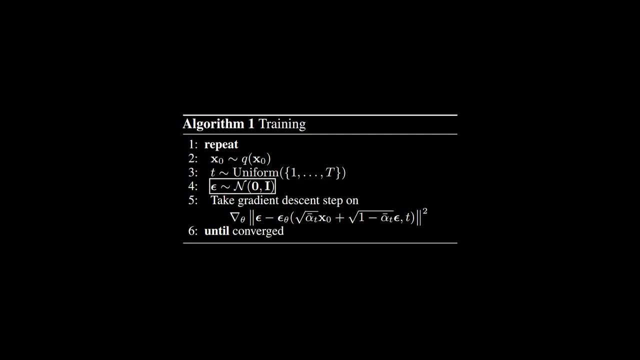 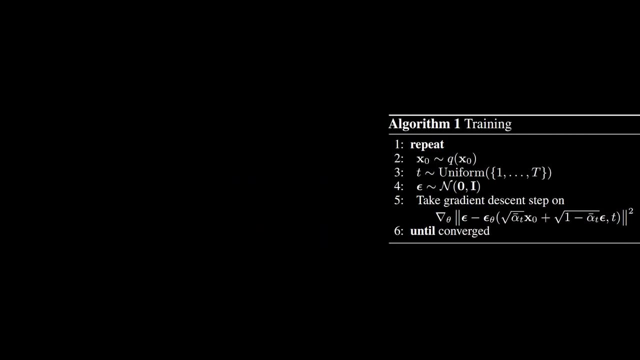 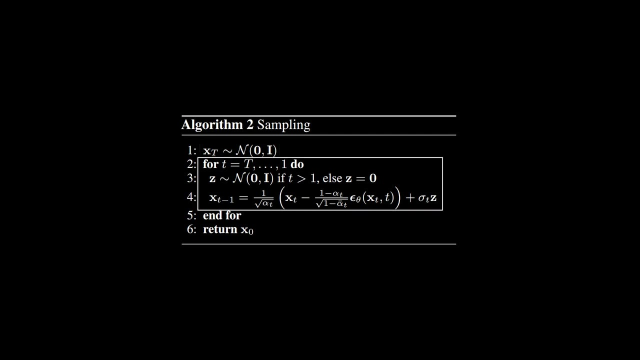 dataset, Then we sample T and we also sample noise from a normal distribution And then we optimize our objective via gradient descent. Super easy, right Sampling is also not that hard. We first sample XT from a normal distribution. That's our starting point, and now we iteratively use the formula which I already showed before. 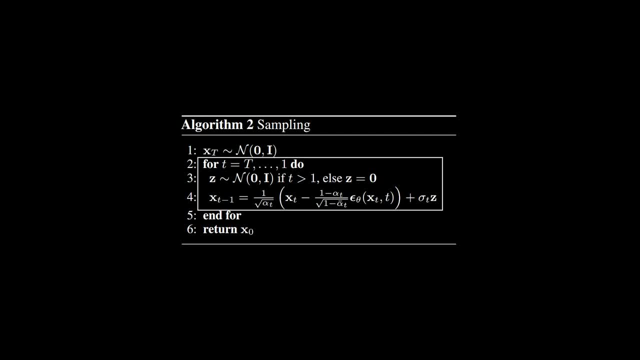 that uses the re-parameterization trick to sample XT-1.. And here you can see how the case for T equals 1 is approximated. If T is equal to 1, we don't want to add noise. Why, Let's imagine we would add noise. 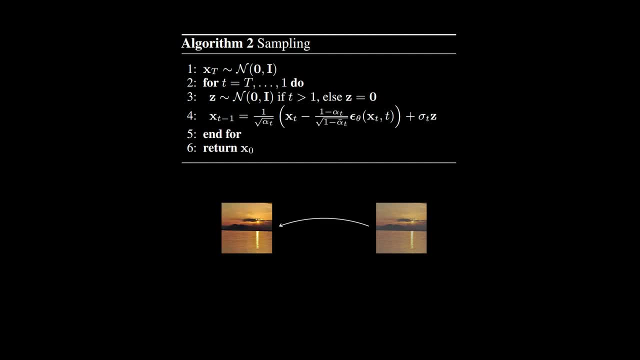 If T is equal to 1. We are predicting X0, given X1. Our neural network predicts the noise in X1, and then we subtract it from X0. Now it wouldn't make sense to add more noise, since we are at our final image and the additional 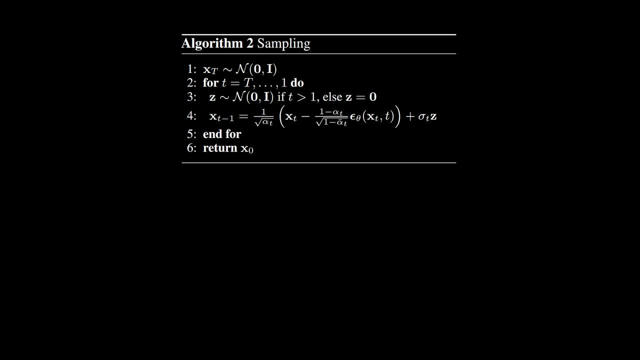 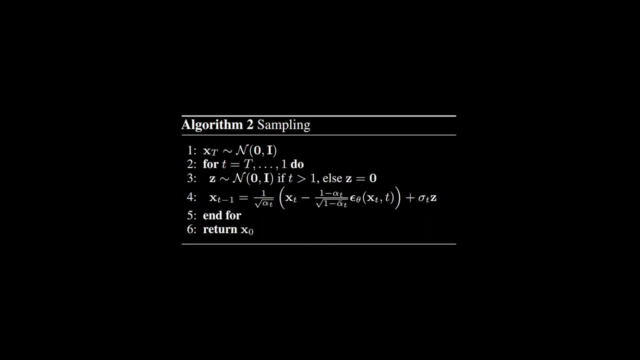 noise would make the quality of X0 worse. So yeah, that's the simple reason and eventually we are returning X0. And if we trained well, we now have an image which could come from our dataset. So you made it. We are done with the fundamental part of diffusion models. 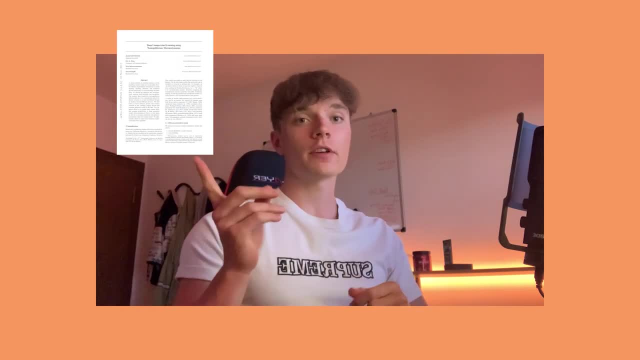 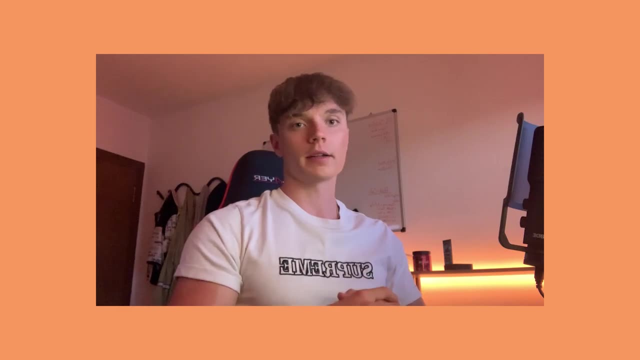 Great job. The last thing we explained was taken from the 2015 and the 2020 paper. Now we already said that there were more improvements done by the follow up papers from OpenAI. I'm quickly gonna show the updates which they made, but I won't go into the details. 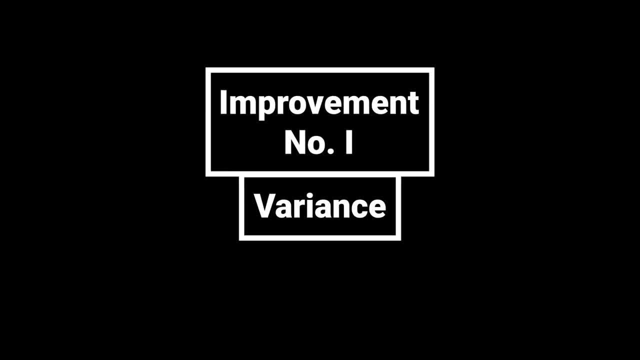 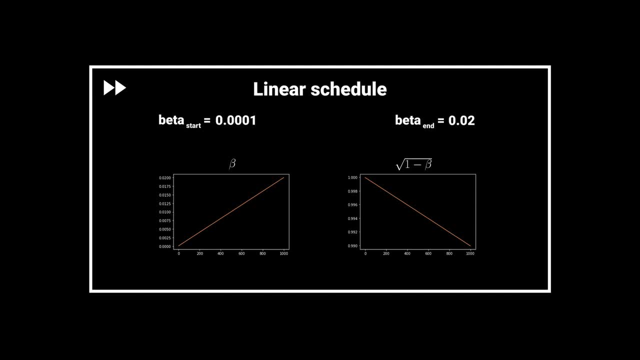 for time reasons. The first improvement is reconsidering the variance Before we just fixed it to either beta or beta hat, which are the upper and lower bounds on the variance. Now we are also going to learn it. Specifically, we are learning an interpolation between beta and beta hat using the following: 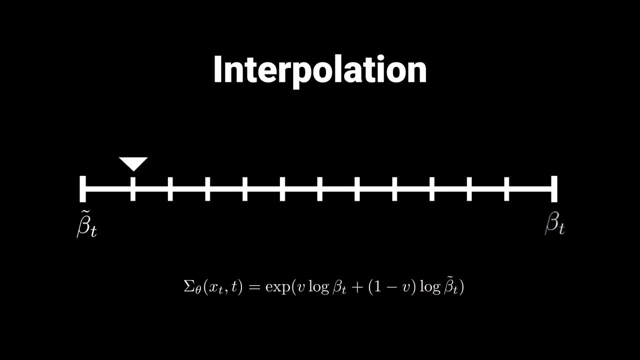 formula. The authors just found it to work better than to learn it directly, because these numbers are in a really low range. But now we just need to learn a number between 0 and 1, which works quite well. This also results in a slight change of the loss, since it doesn't depend on the variance. 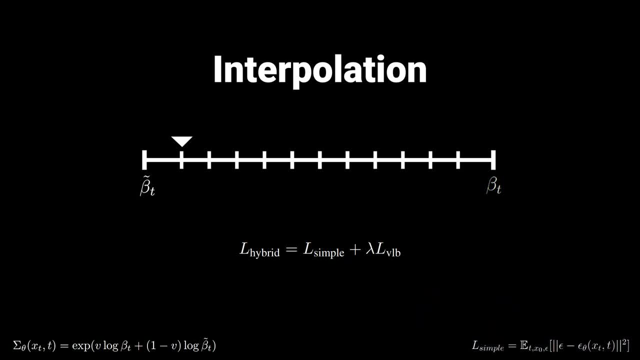 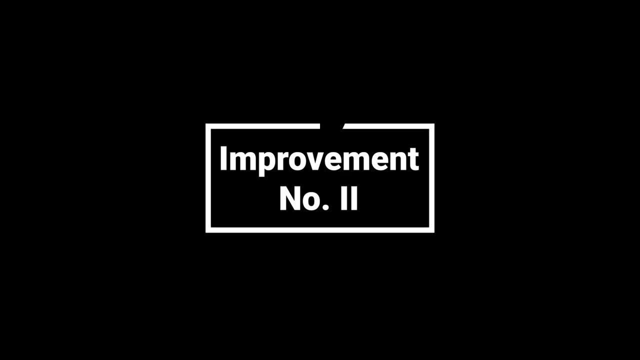 in its plain form. We add the variational lower bound to our loss and scale it with lambda, which was defined as 0.001.. Next up, it was also proposed to use a better noise schedule. The new proposal doesn't look as simple anymore. 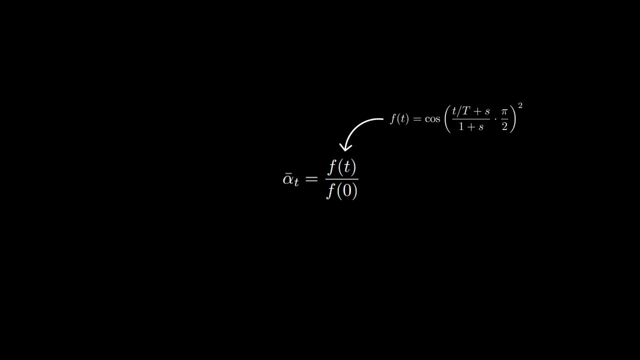 It is as simple as the linear and is defined by the following formula for alpha hat, from which we can derive beta. Here you can also see what it looks like when we plot both schedules. It was designed to have little change at the extreme points at the beginning and at the 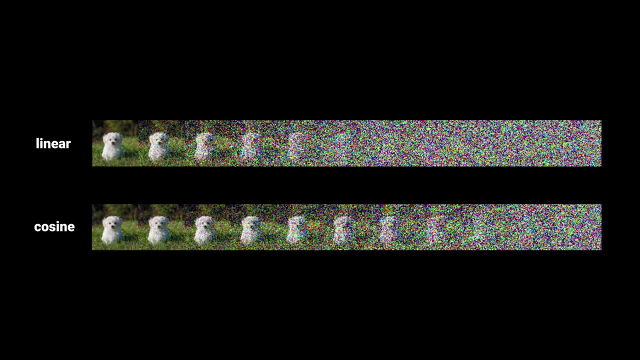 end and to be linear, in the middle region, And I have shown this figure before, but once again you see that the cosine schedule behaves better and takes more time for destroying the information in the image. Make sure to check out the paper to get more explanation on their improvements and other. 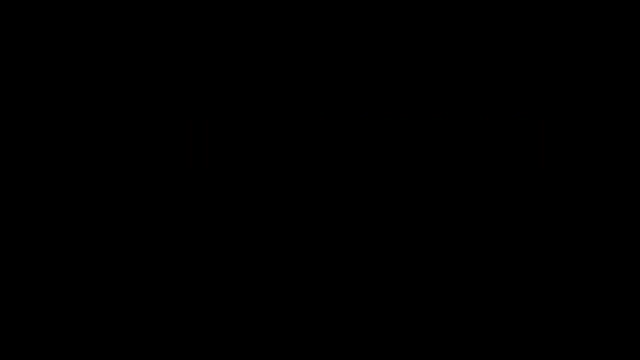 things. And now for the last part, let's quickly take a look at the results of the papers. Specifically, I want to take a look at the FID scores of the different diffusion model papers and also compare it to other non-diffusion models. 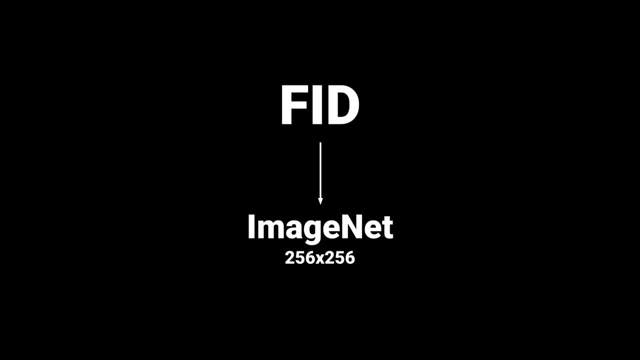 Here I will only look at the scores on ImageNet 256x256, but feel free to check out all the papers to see different data sets and also other metrics such as bits per dimension. Unfortunately, the 2020 paper hasn't trained on ImageNet. 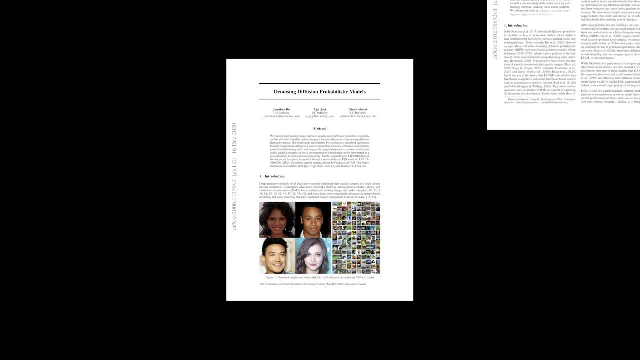 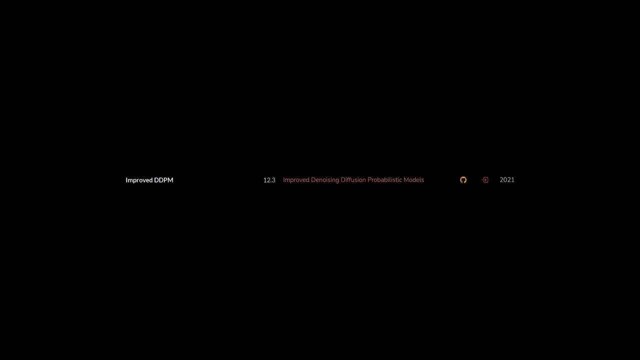 But it obviously has a lot of data. So let's take a look. ImageNet would perform much worse than the improved diffusion model, which outperformed it in all other categories. The improved DDPM achieved a score of 12.3 on ImageNet. 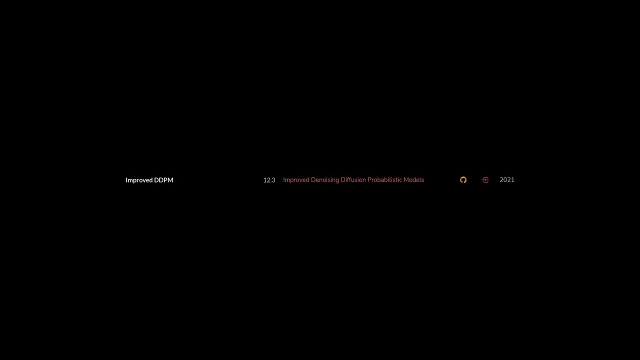 That's quite a good result, but the improvements from OpenAI completely outperformed it and achieved an FID score of 4.59.. By the way- and ADM stands for ablated diffusion model- Later in the paper, they also proposed a technique for upsampling in the diffusion process, which 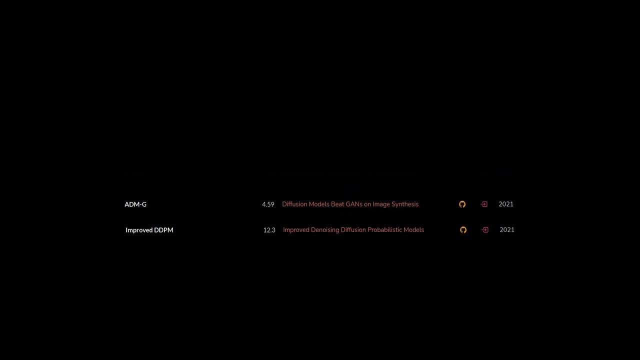 I didn't talk about in this video. With that, they improved even more And achieved a score of 3.94.. These results are incredible, but let's take a look at how diffusion models compare to other models. You see that the improved DDPM ranks last among all these state of the art models. 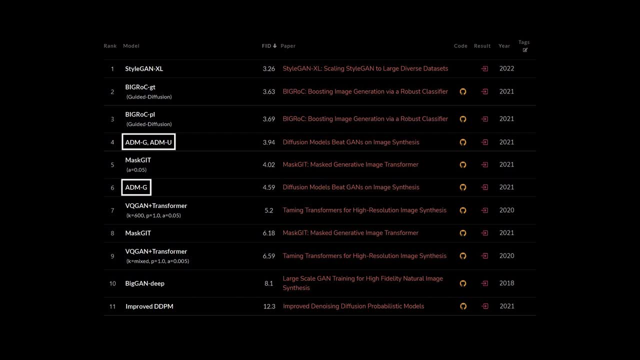 However, the approaches from OpenAI are placed 4 and 6.. And, even better, the results from the paper BigRock, which is also a diffusion model which I didn't cover in this video, rank even higher, with an even lower FID score. 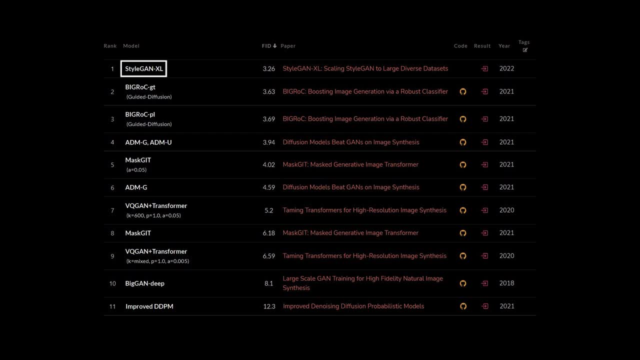 But still the gold medal is being hold by a GAN paper with some margin, Although I believe that diffusion models will easily outperform GANs in the near future. We've been working so long on GANs to get them working, and diffusion models have just. 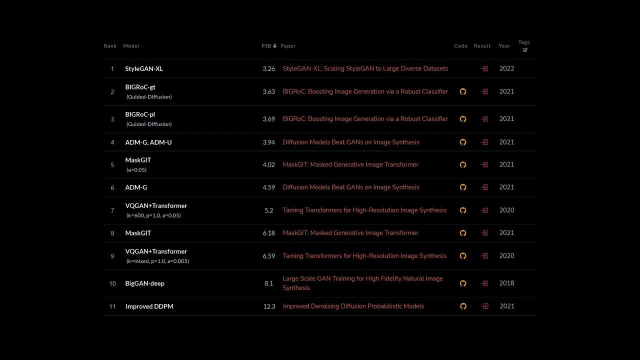 recently rise and not much effort has been going into its research, So I'm definitely excited where all of this will be going. Also, let me know if you would like to have a video about any of the other papers listed here. For example, last time I already did a video about VQGAN. 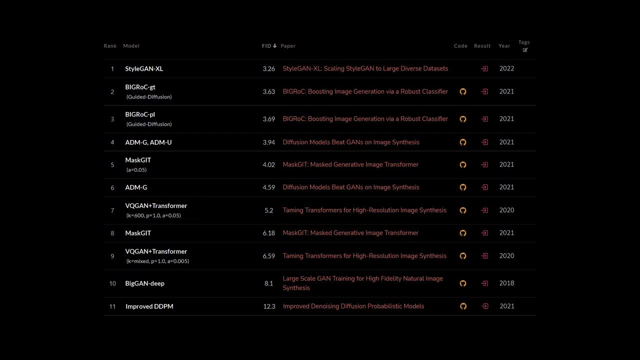 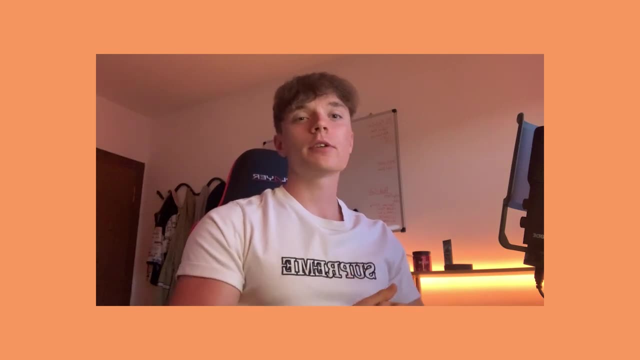 Check it out. if you want, then also feel free to suggest other papers which aren't listed here. And finally, we are done Great job if you followed all the way until here, But don't worry if you didn't understand every single part. Therefore, let's quickly do a recap so you take out the most important things of the 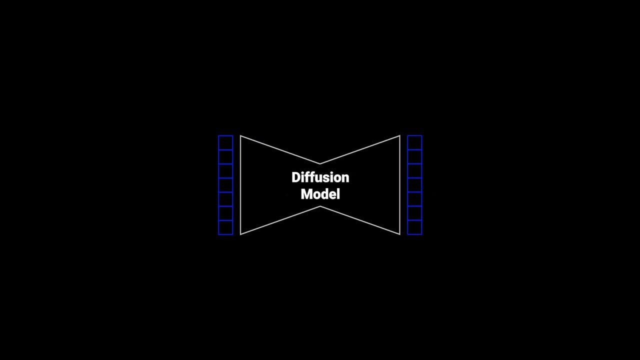 video. Diffusion models are generative models which became super popular in recent times for beating GANs on image synthesis. The main idea behind diffusion models is that we have two processes. The first one is easy: we just gradually apply noise to an image over a lot of steps, until the image has turned into concrete. And the second one is very easy: We just gradually apply noise to an image over a lot of steps until the image has turned into concrete. And the third one is very easy: we just gradually apply noise to an image over a lot of steps until the image has turned into concrete. 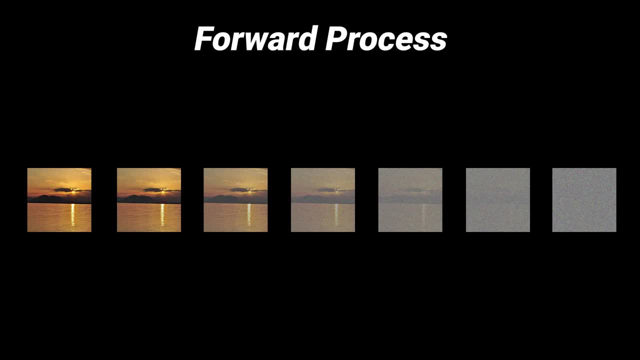 And the fourth one is very easy. we just gradually apply noise to an image over a lot of steps until the image has turned into concrete. The cool thing is that we can also do this in one single step, which saves us a lot of compute and time.